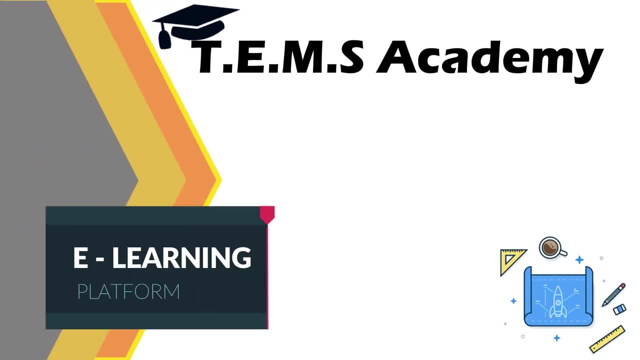 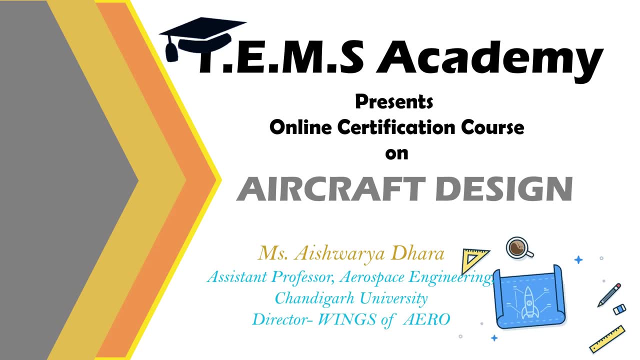 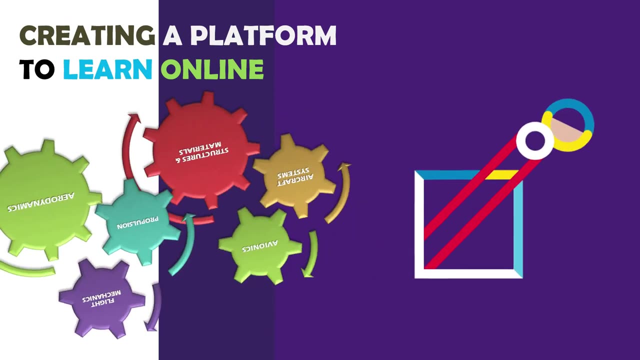 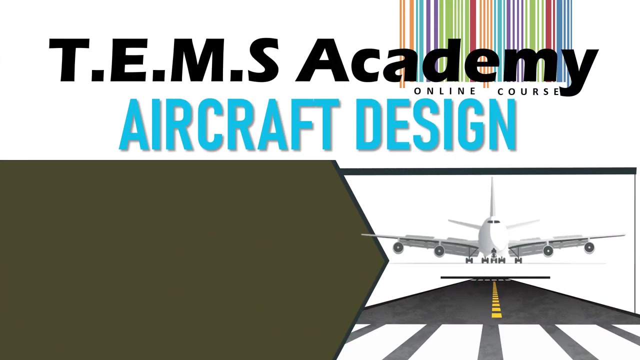 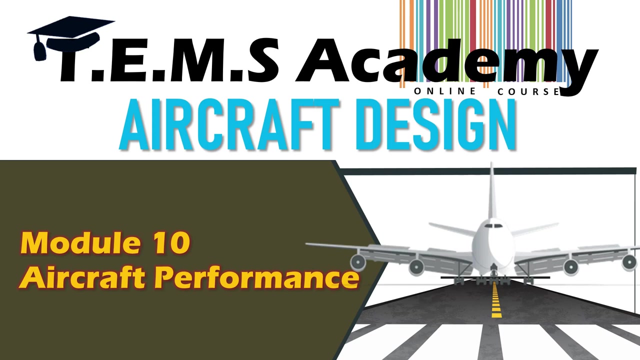 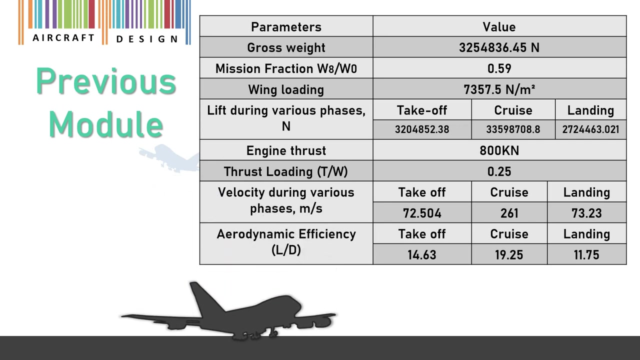 hi friends, welcome back to aircraft design module 10: aircraft performance. this video will give you the clear conceptual details about the phases of aircraft performance, from takeoff to landing. in addition to the aircraft designer point of view, special highlights will be given for non-powered aircraft and electrical propeller or electrical powered aircraft. 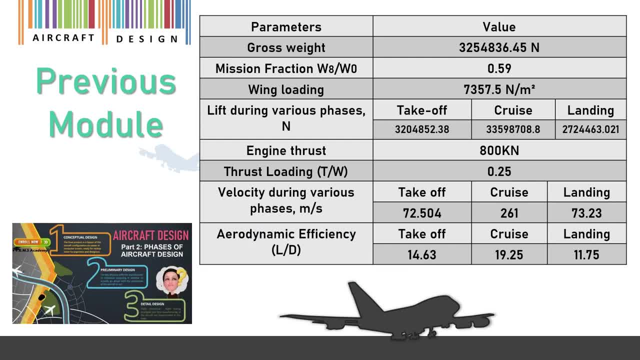 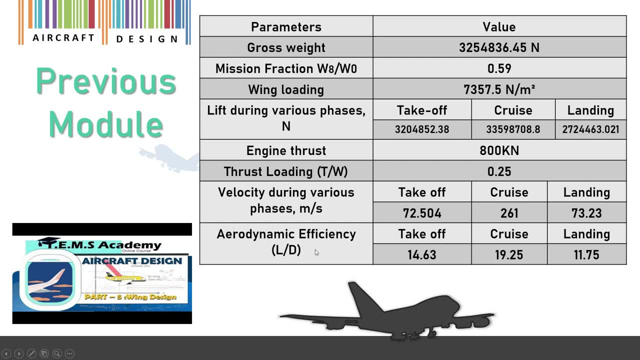 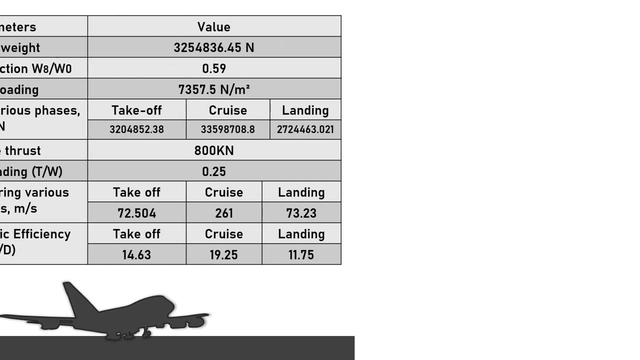 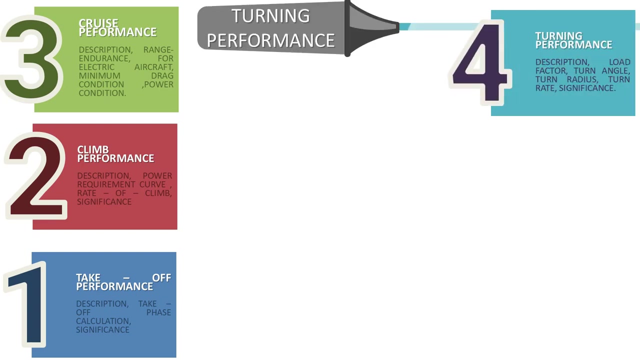 so far the previous aircraft design module- these are the following details- has been obtained, with estimation to each aircraft components, design and sizing. to the drag estimation today we will see one of the most important aspects in aircraft performance includes tick off, climb, cruise, turn, descent and landing considering 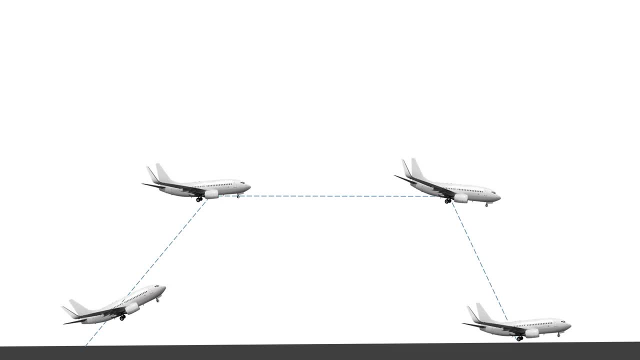 all of the principal components of flight performance involves steady state, flight conditions and equilibrium of the aircraft. make a note that a proper prediction of aircraft performance is an important step in the entire design process. so performance and payload are what which will sail an aircraft more than anything else. 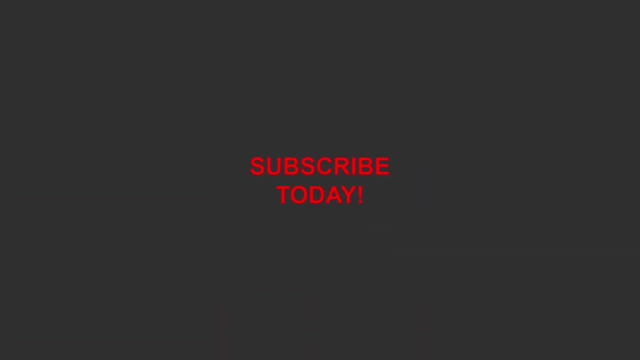 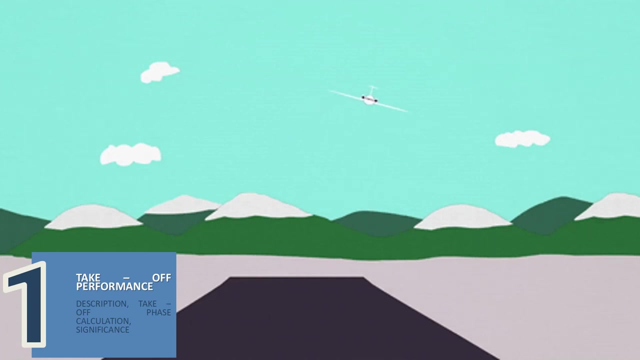 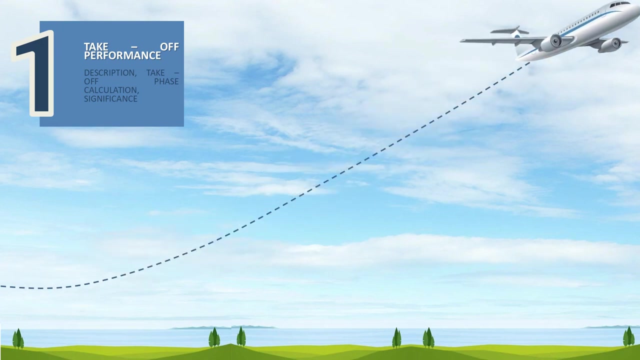 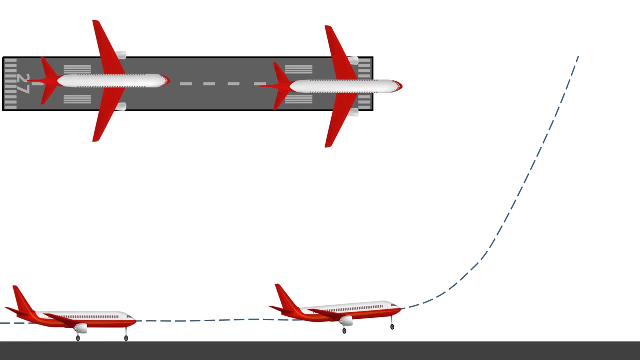 so when an aircraft becomes airborne, it must take off from the ground or, as a muchos nueva era, known as avionics. does an aircraft takeoff from the ground or sea? so when an aircraft becomes airborne, it must take off from the ground or sea. now aircrafts primary. 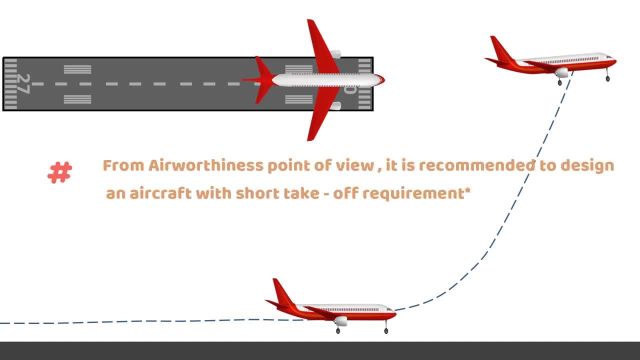 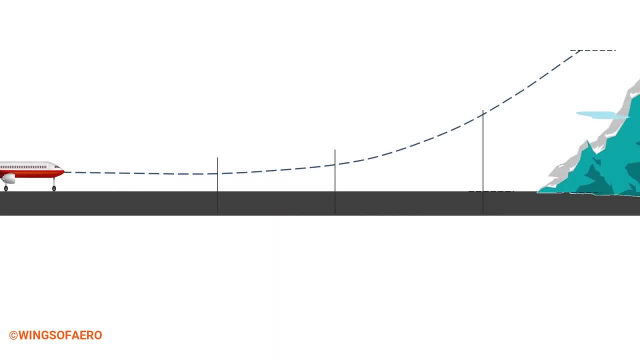 from the airworthiness point of view, it is recommended to design an aircraft with a short takeoff requirement. okay, so we will see what is mean by takeoff. takeoff is a distance required for an aircraft to accelerate from zero velocity to the takeoff speed and climb over 35 feet to. 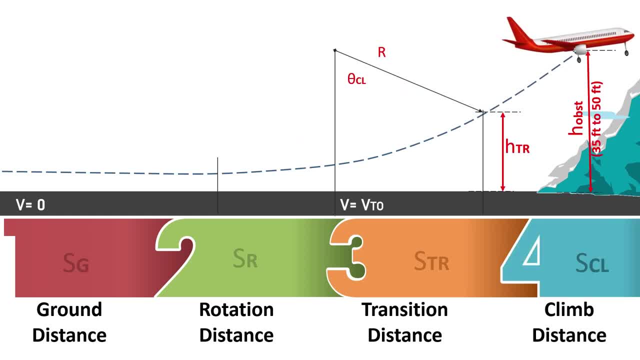 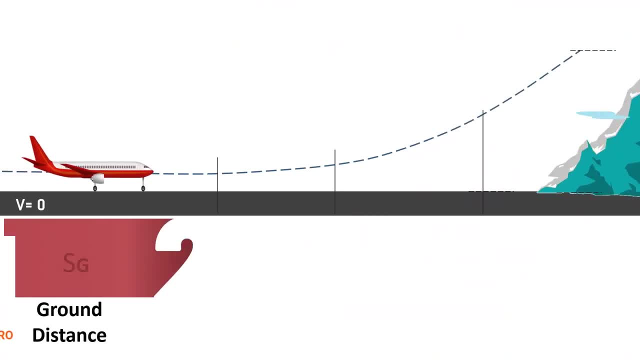 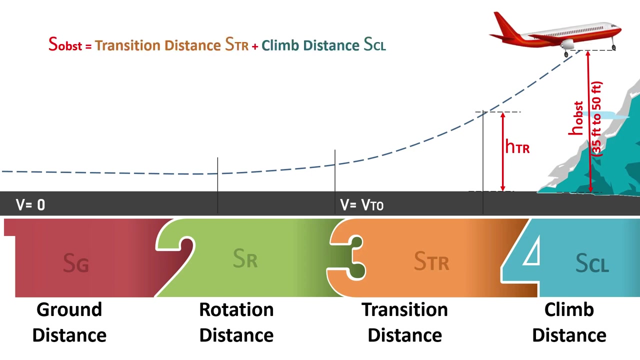 50 feet of struggle. in case of military and for the commercial aircrafts now, takeoff distance is a sum of ground distance, SD, rotational distance, SR, transition distance, STR and climb distance, SCL. combination of transient and climb distance is also expressed as obstacle distance first determine. 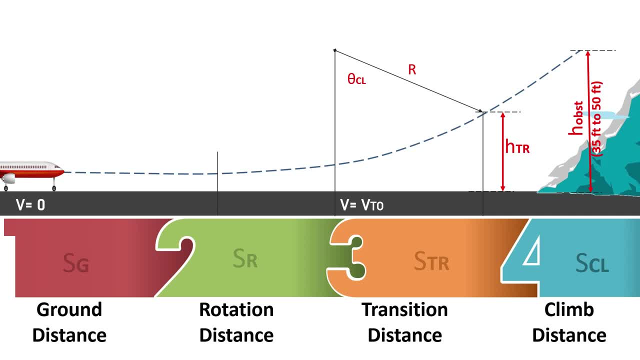 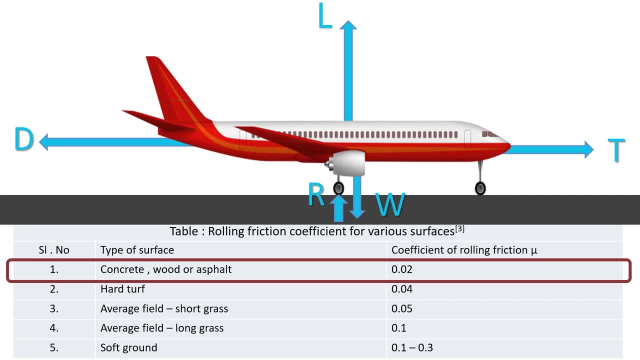 the takeoff ground distance and climb distance and then the takeoff distance and then the takeoff ground run. it starts from rest and accelerate to the takeoff speed. that is VT, not the forces acting on the aircraft during ground run, that the ground reaction are and the rolling friction mu are, and 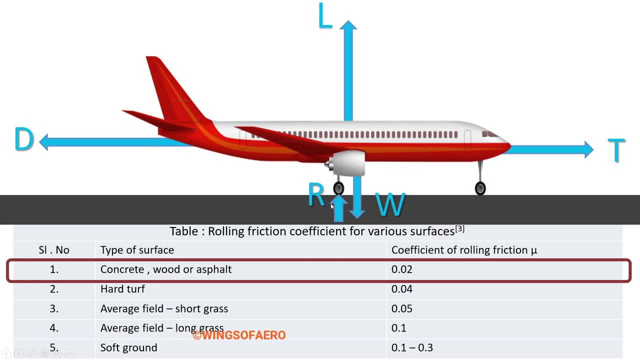 additional forces: lift, drag, weight and thrust. now mu is the coefficient of rolling friction between the runway and the landing gear wheels, because the runway surface differ from one runway to another, like pave level, smooth and dry runway surfaces. in case of military and the commercial aircraft, concrete to be chosen. so in my design, concrete is. 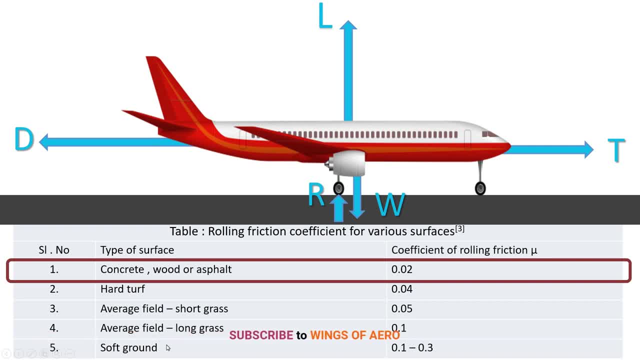 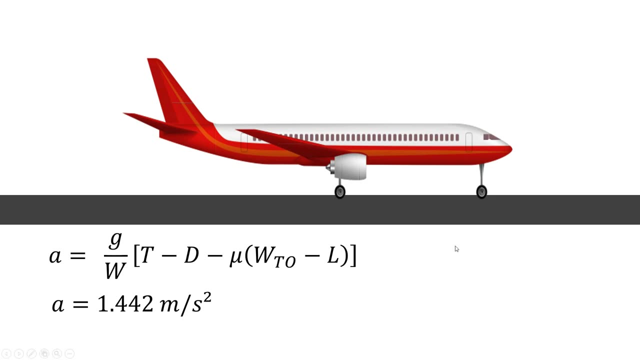 to be chosen. so based on the type of aircraft or the runway, this, based on the stable parameters will be. new value will be chosen. so the equation of motion becomes, that is, W by G, into a acceleration mass, into acceleration equals to the force. now, what are the forces? are there? 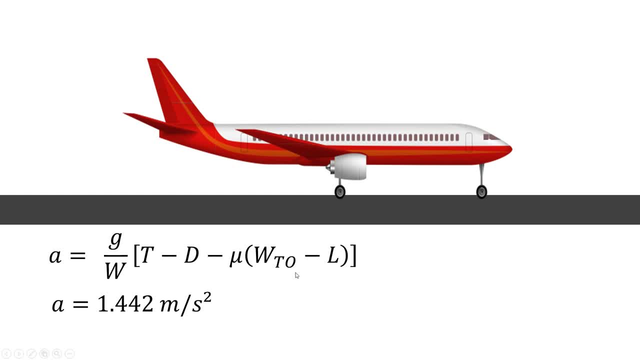 based on this forces. we can write this equation now. here mu is chosen as 0.02. now, after solving the substituting the values, we get a equals to 1.442 meter per second square. so therefore, remember one more thing: in case of propeller driven, we need to use 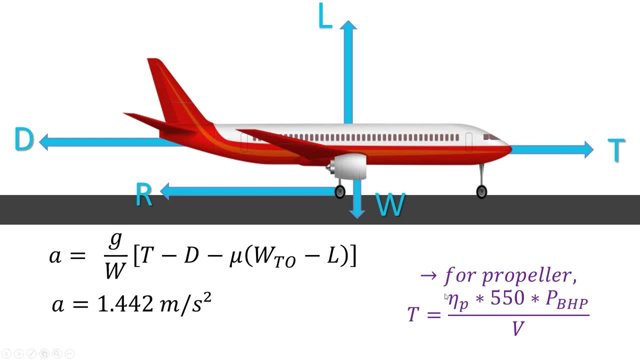 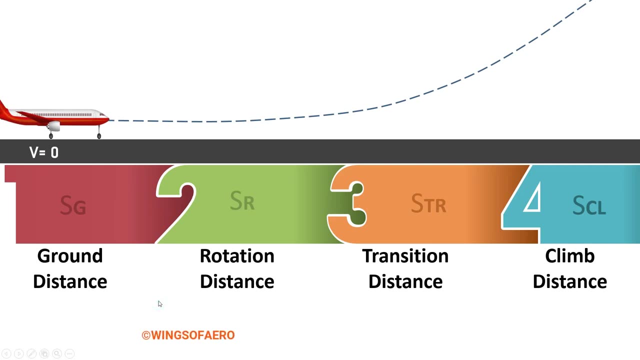 the formula to find the eta depending on the fixed speech, climb, cruise and constant speech. right, okay, coming back to this, the ground speed. so therefore, the ground speed is defined as the takeoff speed square to the twice of acceleration. now, takeoff speed is all already found, that is. 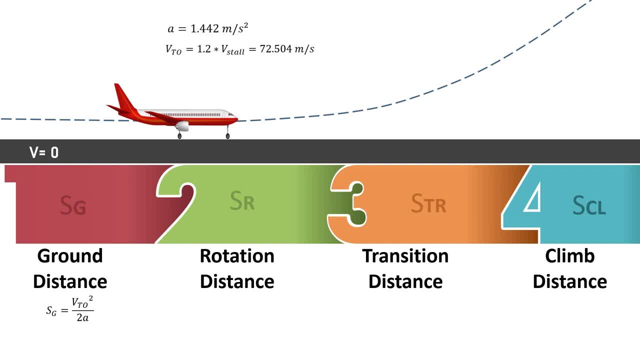 seventy two point five zero four meter per second. substituting the value we get the ground speed is speed about 1822.462 meter. now coming to us: rotational distance sr is a distance in which the aircraft's nose wheel is off the ground and the pilot pulls the stick back and increase the. 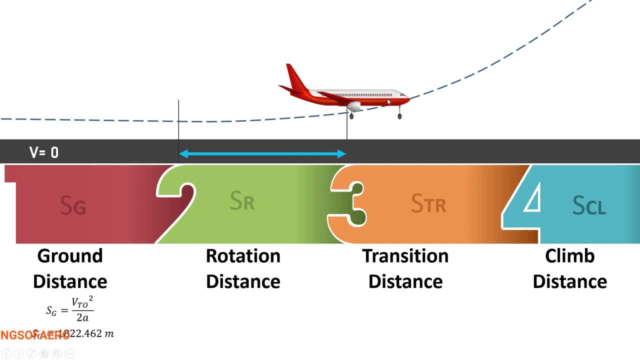 angle of attack of the aircraft. as the speed increase or exceeds the takeoff speed of the aircraft gets the airborne so the main landing gear wheels leaves the ground at this particular stage. so, based on faa regulation for commercials, for small flight, military and large passenger aircraft, based on this following time limits you can find, as you can see here, for small sr equals: 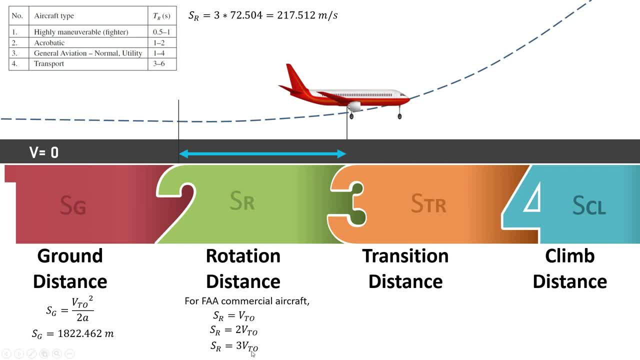 to v? t naught. in case of military, usually it has been taken as two. second. that is esimerk적으로 for small. sr equals to vt. in case of military, usually it has been taken as sr equals to 2 into vt naught and in case of larger transport or cargo aircraft it's been 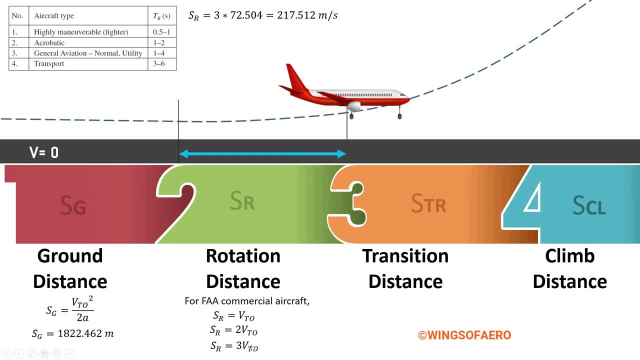 considered as 3 vt naught. so in my design we'll be considering the 3 vt naught and we will get the rotational distance about 217.512 meter. now, determining the obstacle distance is the summation of the transient distance, str, and the climb distance, scl, as shown in figure. now this: 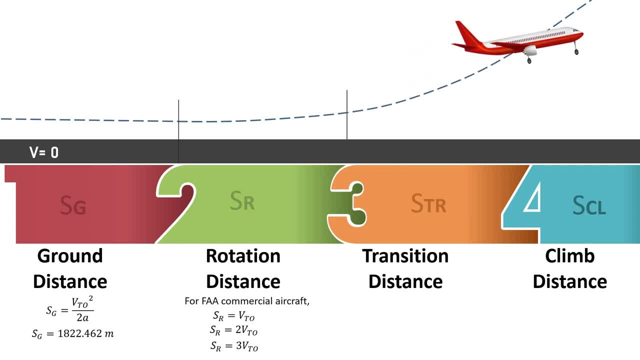 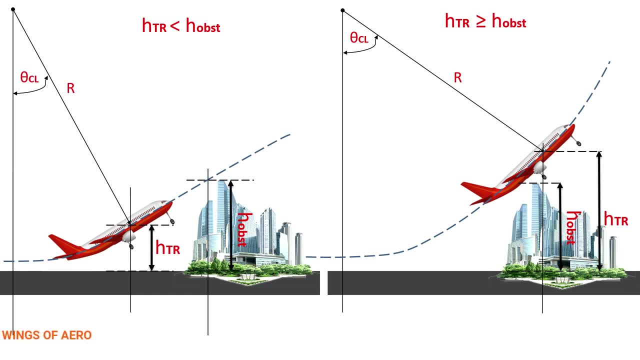 obstacle distance depends on what is the height of the transient height and the obstacle height. now if, in case this htr, that is, transient height, is greater than the obstacle height, okay, obstacle height are generally considered as 35 feet to 50 feet, so in case of larger transport or cargo aircraft it's been considered as 3 vt naught and we will get. 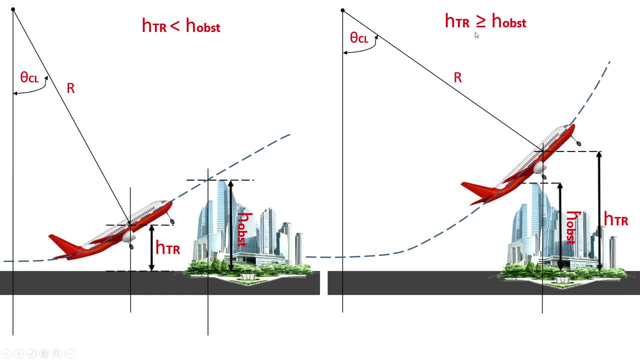 so in that case what happens? the str is equals to s abstract, as shown in figure, where scl becomes zero. but if in case okay, htr, that is a transient height, is less than the obstacle height, then the obstacle distance can be find by summation of transient height. 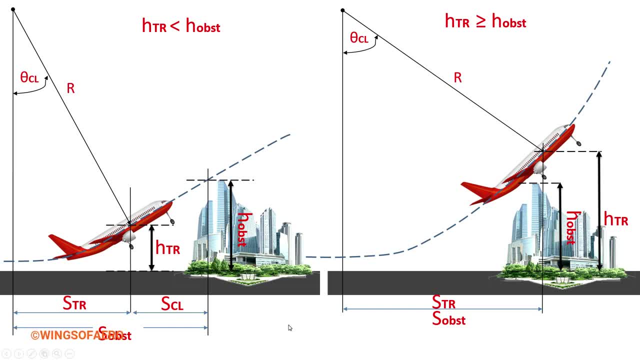 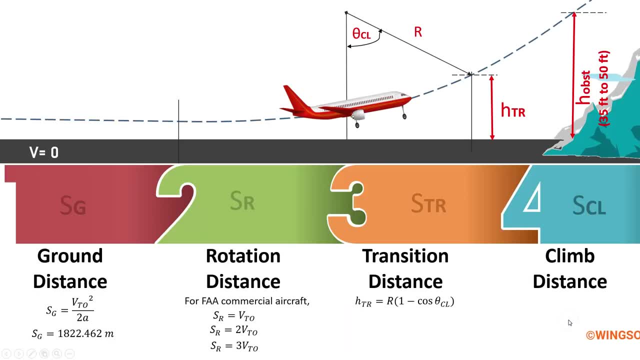 plus the climb distance, so as you can see here. so first let me find the height of the obstacle height and then the height of the climb distance, so we will find the transient height, that is htr. now htr mathematically can be find using this formula: 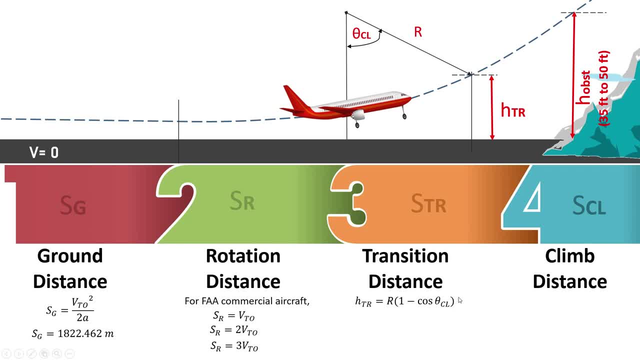 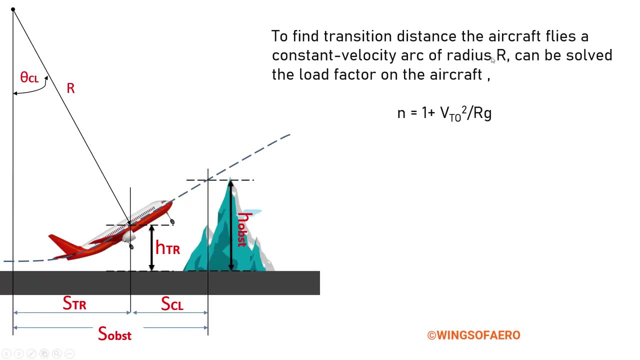 r 1 minus cos, theta cl. theta cl is the climb angle. okay, r is the radius of arc at what distance it is climbing. so to find out the transient distance, the aircraft flies at constant velocity. arc of radius r. now it can be solved using the load factor. 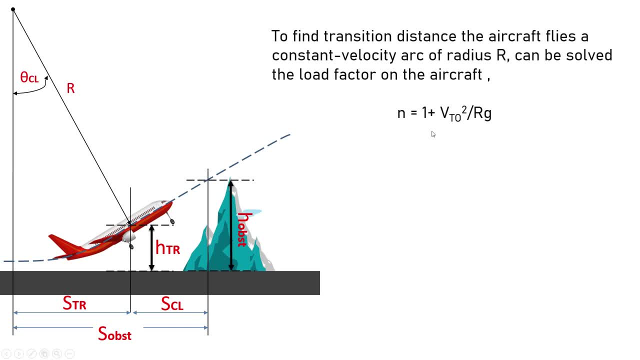 of the aircraft. that is n equals to 1 plus v t naught square by r, g. now v t naught is also known to us and g is also known to us. now we need to find the unknown. that is n and r, now n can be. 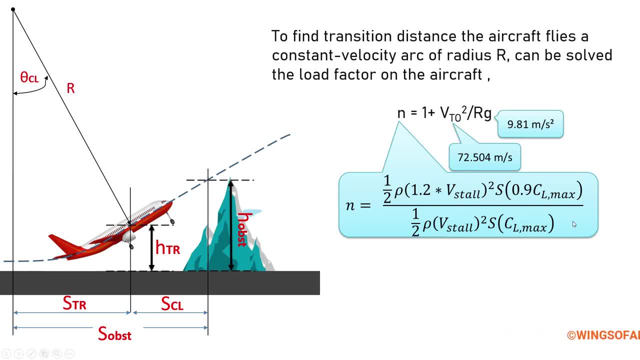 find, using this load factor during the transitions, using this formula, applying the formula, we get in about one point two, nine, six. now we know in all the parameters and substrates we know that the values we are substituting in the r formula, we get r about one, eight, one zero point three, five, three. 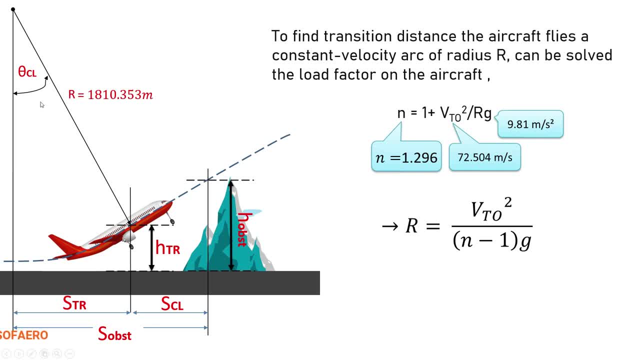 meter. now, same goes for the climb angle. climb angle equals to sine inverse of t by w minus one by l by d. during take off. now, again applying the values, we get the climb angle to be around 10.47 degree. now, finally, substituting back in the transient height formula. after that it is going to. 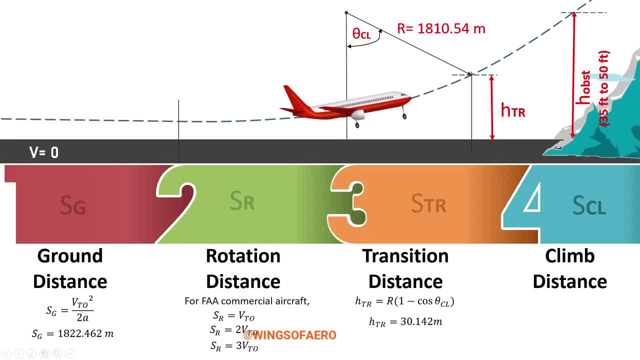 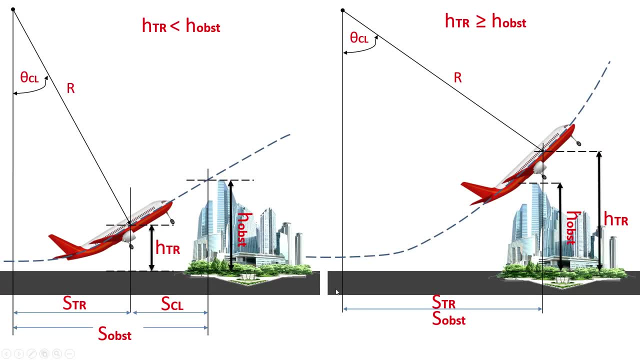 be 10.47 degree. so it is going to be one from one and the second one is going to be about an four substituting and resolving. we get as 30.142 meter. now it says that it, that is, transient height, is greater than the obstacle height. so here, in this case, in case of my design, the transient height, or 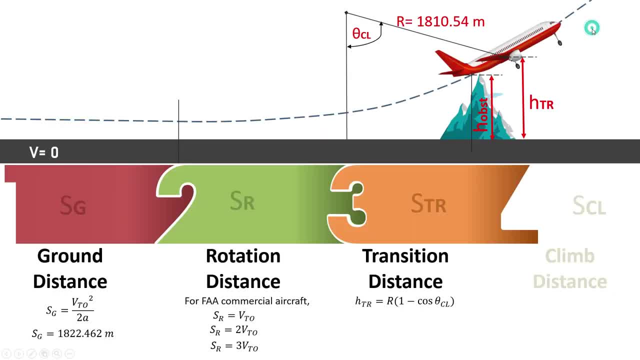 the transient distance is equals to the obstacle height, where the climb distance will be zero. and the transient distance can be find using this formula: r sine theta cl. so we know all the formula and when substitute we get 3 to 8.98 meter right. so in case of my design, total takeoff distance can: 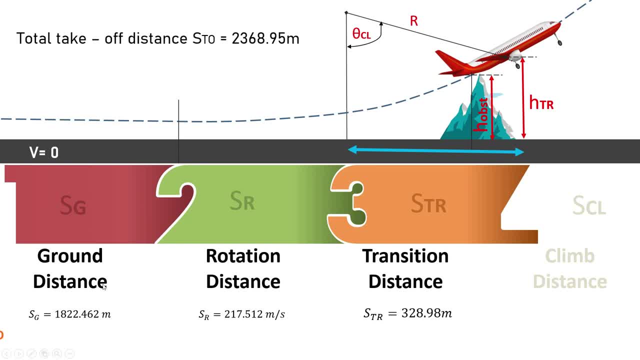 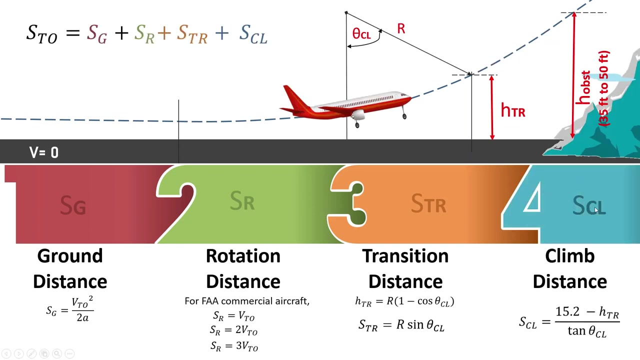 be find the summation of all the three parameters, that is, ground roll distance plus rotation distance plus the obstruction distance. summing up we get about 2368.954 meter total takeoff distance. but in case of your design, if it is htr, that is, a transient height is less than the obstacle height, then s climb can be. that is. 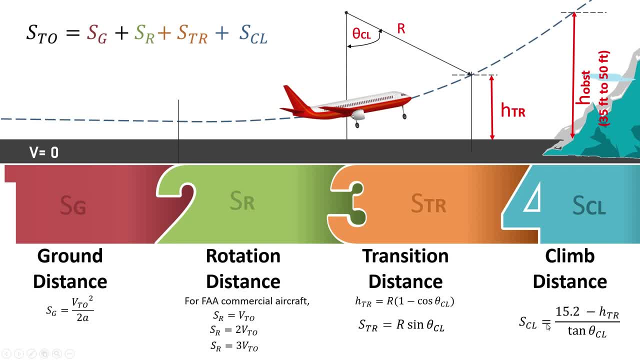 a climb distance can be find using this formula: 15.2 minus hdr by tan, theta, cl. so htr is also traveled for a long distance and the buckling distance is less than the obstacle height and an known for you. theta is also known for you and remember, this is in terms of meter. okay, now here. 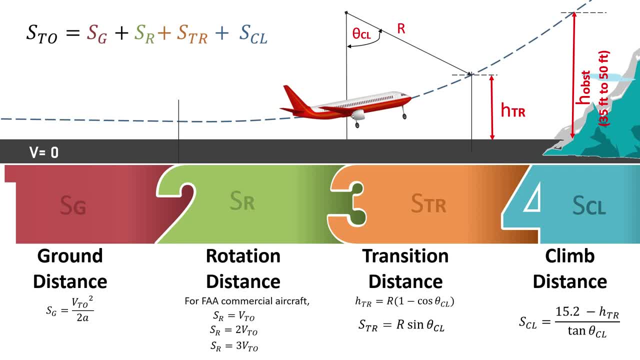 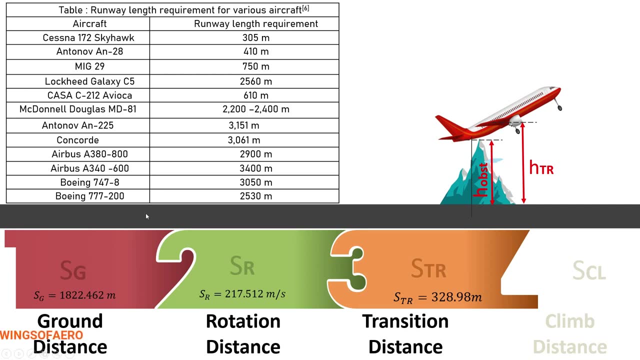 to find out the total distance, it will be sum of all the four parameters: sg plus sr plus str plus scl. to find out the total takeoff distance. i will check the landing and takeoff distance of my reference aircraft for an example. boeing 777, okay, has an um takeoff distance about 2530 meter, okay. 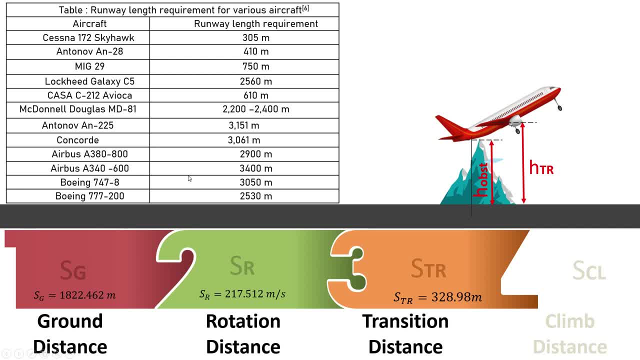 and considering this 340 variant or those takeoff distance also 3400 meter, so you can find the significant good takeoff performance. so as we need the less takeoff distance, better the performance. now, if suppose you are exceeding the limit, then you need to check your parameters, especially the thrust. 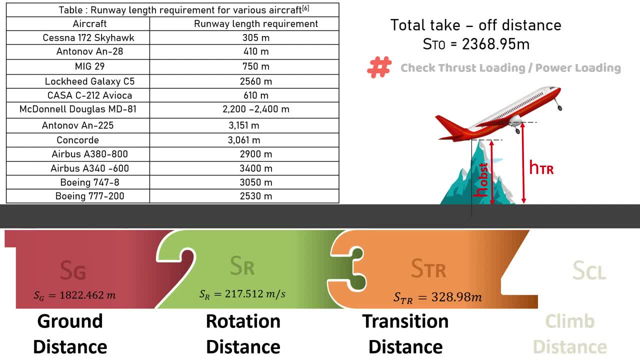 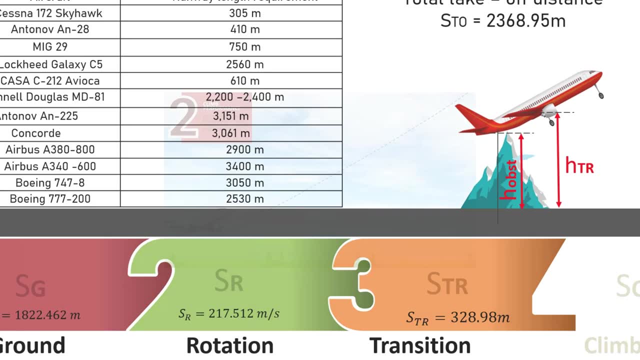 loading, that is t by w ratio. or, in case of propeller driven, you need to consider the power loading, that is p by w ratio, because takeoff is a function of acceleration and speed. okay, now, takeoff maneuver is followed by the climb maneuver, which is the vital for aircraft designer. 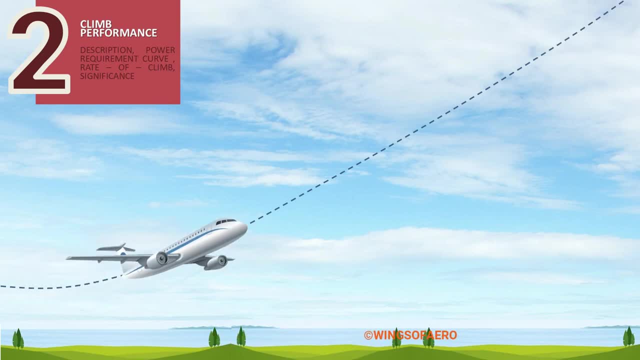 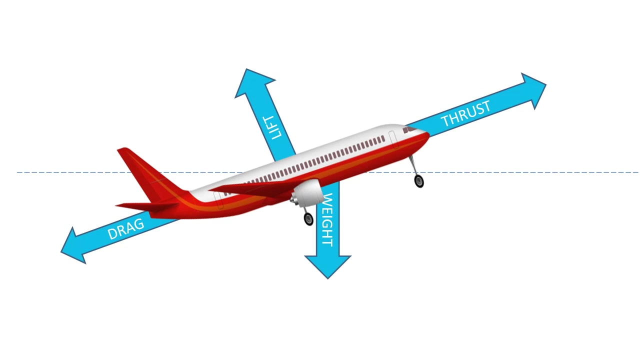 to understand how rapidly or how steeply an aircraft can climb, so greater the climb performance cells the aircraft. so study of climb primarily involves the determination of the rate at which the aircraft increases its altitude. that is a rate of climb and the angle of flight path makes to the ground. it's okay. so the angle of climb, as you know, as you can see in the figure, 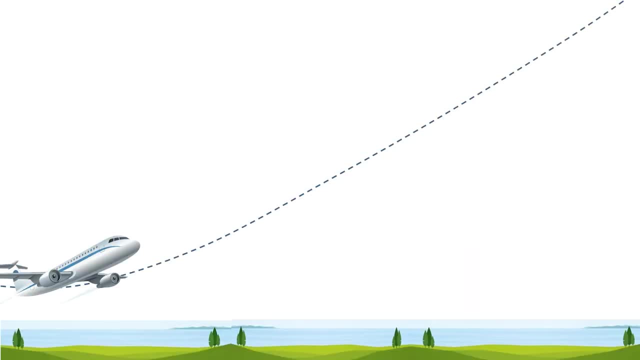 we find, using the rate of climb, equals to the power available minus the power requirement by the total takeoff weight. okay, so, uh, the power available is estimated by multiplying its thrust by the air speed. as you can see, uh, for my aircraft, and i have done that in my excel, 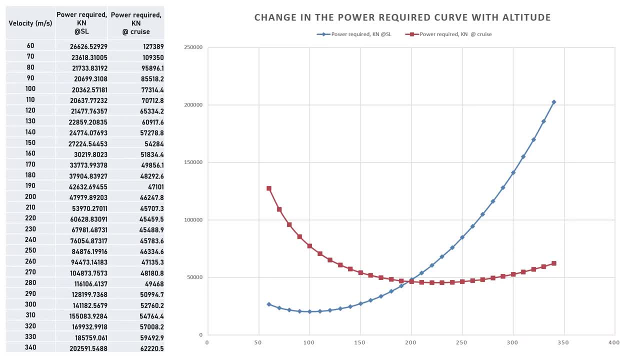 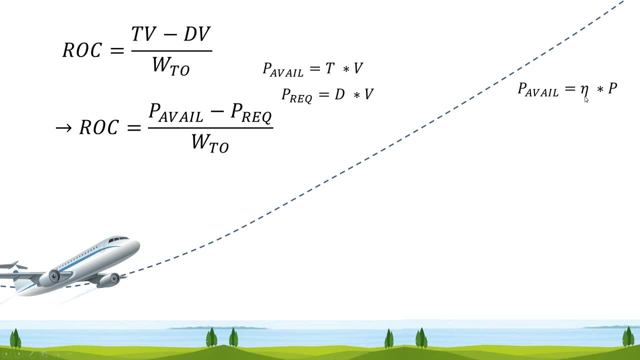 and i have substituted the formula, as you can see, okay, for the various flight speed. so note that. one more thing, for in case of aircraft powered by propeller, the power is obtained by multiplying the engine power by the propeller efficiency. now, if the power in terms of horsepower, the number 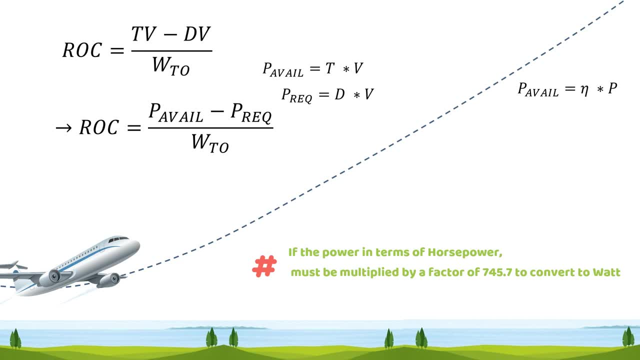 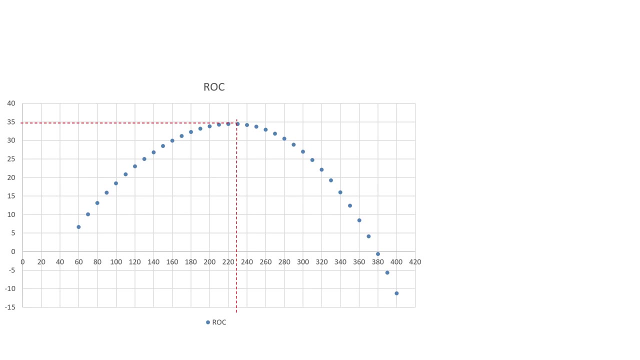 must be multiplied by the factor of seven, four, five point seven to convert to the watt. okay, so from this graph you need to find out this, uh: maximum rate of climb. okay, so, as you can see in this graph. so another thing: to find out the velocity for your maximum rate of climb. also. 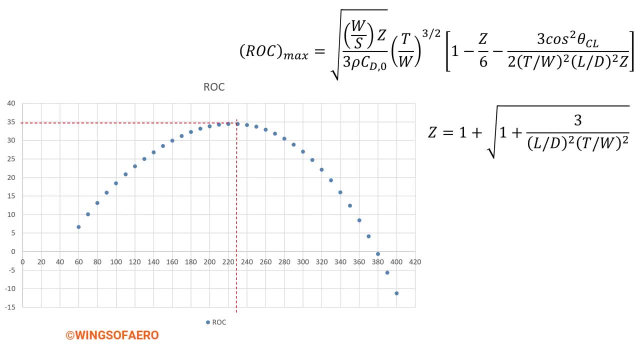 can be fine using this formula. so you can see there's a very complicated formula, right, and after substituting all your known parameters, that is, l by d, t, by w rho uh, w by s theta, cl, cd, naught, okay. so after substituting back, you get your rate of maximum rate of climb about 34.47. 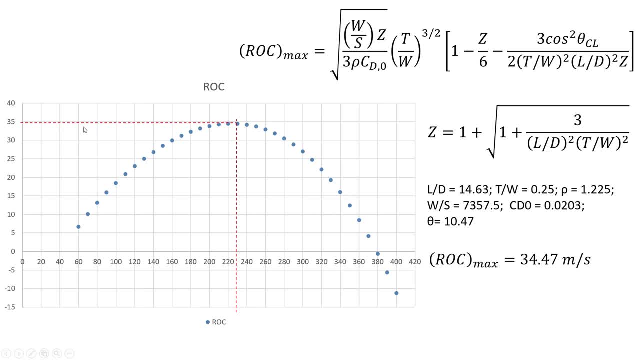 sec per second. even if you follow up in the same graph, you can see the maximum. that curve also lies near 35 meter per second. so you can see this is the completely acceptable one. similarly for in case of propeller driven aircraft, the rate of climb, the maximum rate of climb. 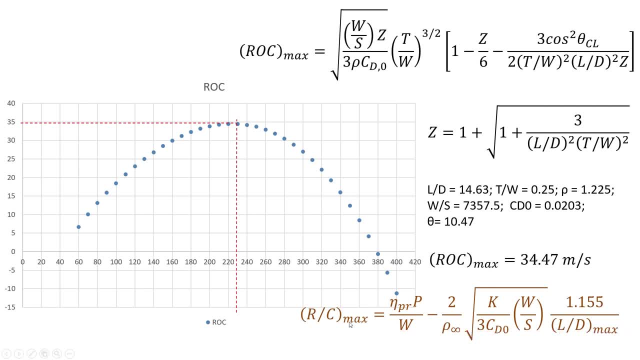 can be also fine using this formula, that is, you can see the here always, you remember, whenever you consider a propeller driven, right propeller driven, there will be some parameter of eta that is based on your propeller efficiency, based on the type of propeller you are using. 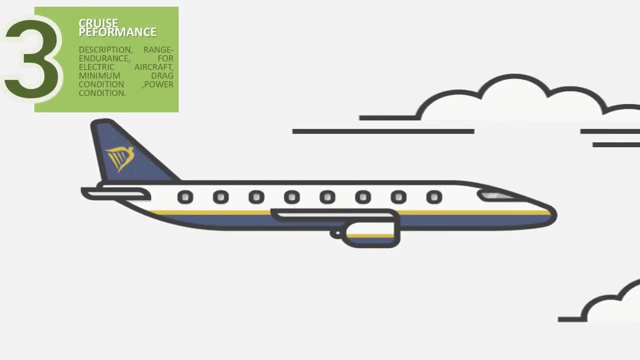 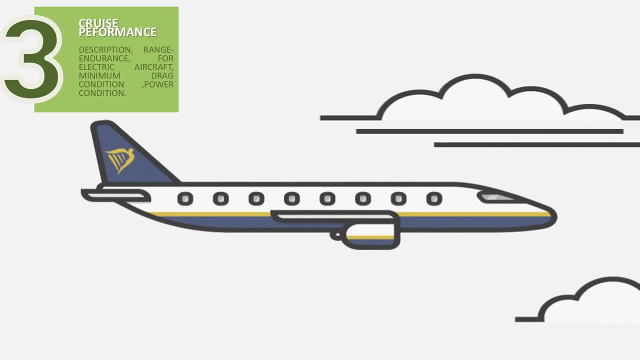 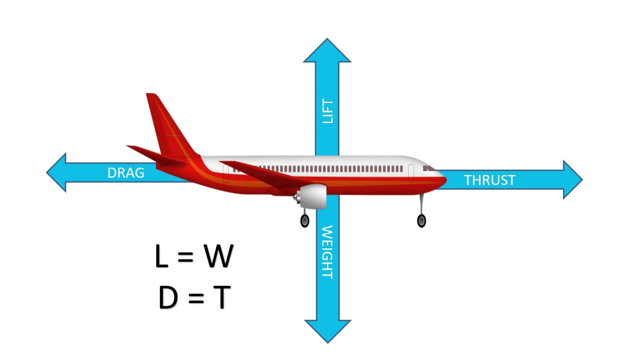 okay, so. so this signifies that the contribution to the positive climb performance in the aircraft- okay now, after climb, move to the cruise- define as a straight and level flight at an constant airspeed. in other words, the strait means the absence of a role which code result in. 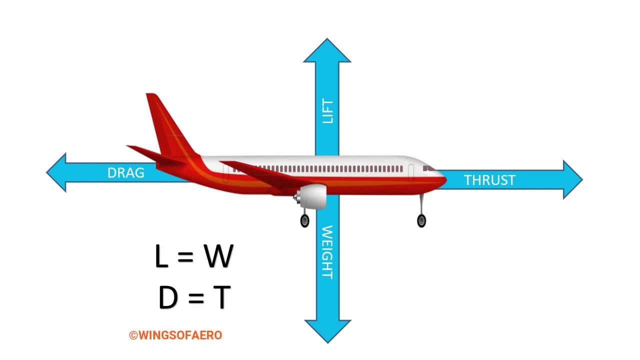 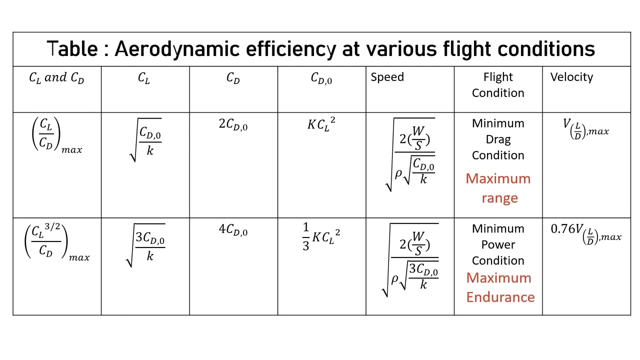 a heading change and level means no change in altitude. assuming the lift is equal to weight and drag is equals to trust. one of the important parameters in the cruise fight is the lift to the drag ratio for the aerodynamic design of the an aircraft influences range and endurance on the aircraft design, whether it's implemented. 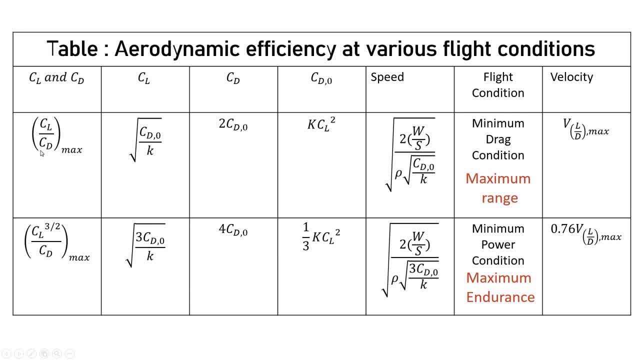 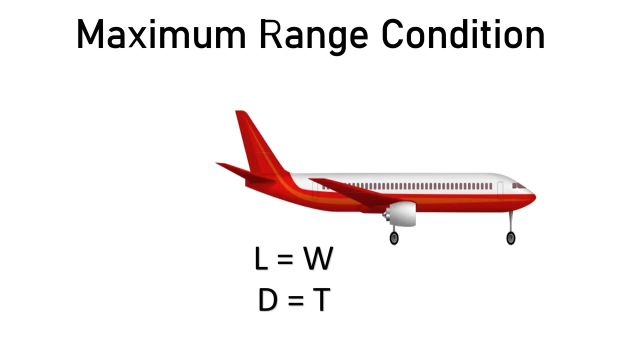 to achieve the maximum range or the maximum endurance. so in case of maximum range, the minimum drag condition is applied, whereas in case of maximum endurance, minimum powered is minimum power required is applied. so the maximum range condition is obtained at maximum lift to drag ratio. okay, so the range is considered is one of the most important parameter in 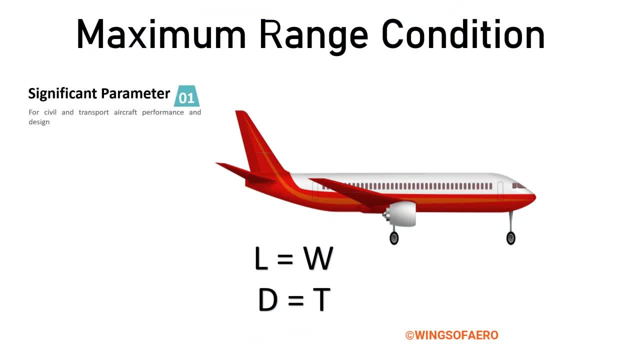 civil aircraft performance and design. now, this is the first priority for the transport jet but the second priority for the fighter. so basically, range is a total distance that an aircraft can fly with the fully loaded fuel tank without refueling. so using the cruise segment is the longest applies the maximum thrust requirement or the drag. 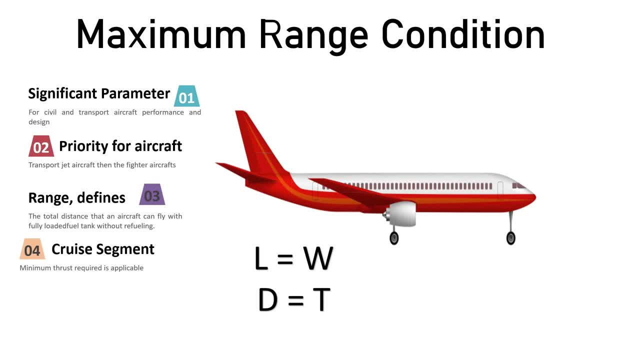 condition. so it is important to note that that for an given aircraft configuration, l by d max occurs at a particular angle of attack and cn, and it is also unaffected by the weight and the altitude. so so the drag determines the thrust requirement, that is tr. tr equals to drag. based on this formula, you can see half row cd. 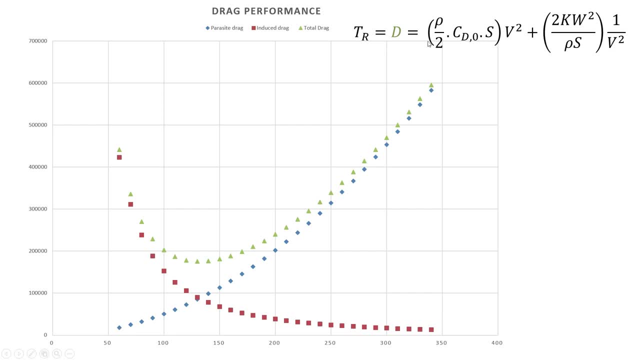 naught into s v square. this is a zero lift track and 2 k w square by rho s by v square is a drag due to lift. now drag and the thrust requirement can be plotted against various velocity as shown in them graph. these are the values for, in case of mine, design, because my design have a different s. 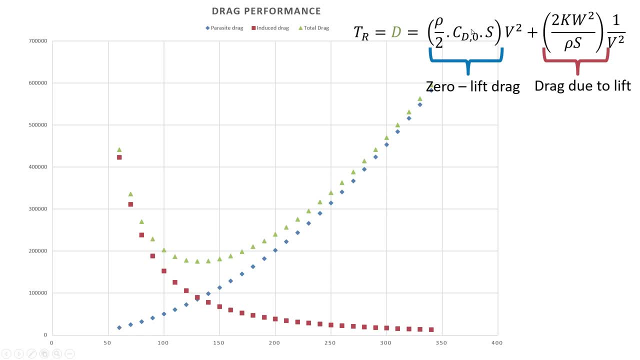 different city knot. similarly, for the k, k is equals to one by pi, e, a, r. this graph signifies that parasite drag dominates at a high speed, whereas the induced drag dominates at the low speed speed. so, based on the certain conditions, we can find out the l maximum l by d. so maximum l by d. 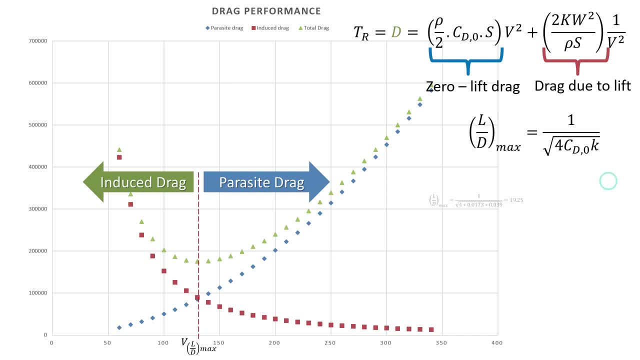 mathematically can be calculated using 1 by root over 4 cd naught k substituting the values. so from there during l by d during cruise can be find that is 19.25 and the velocity for the maximum l by d or the minimum drag condition is expressed as this formula, now substituting the values and: 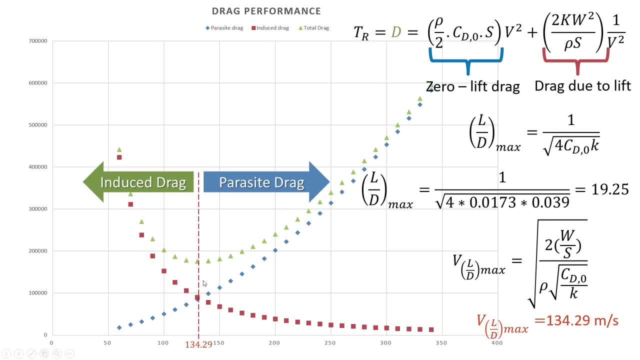 you can get us a 134.29 meter per second and if you observe carefully in this proper graph, you can see this maximum uh, this, uh, this uh l by the velocity at this l by d is almost approaching towards 134.29. another significant aircraft performance and the design parameter is the. 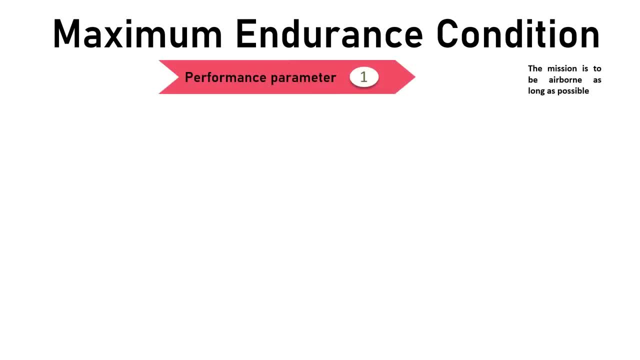 interval endurance. for some aircraft the most important parameters or the performance parameters of the mission is to be airborne as long as possible, that is, should have the long endurance. so the maximum endurance condition will be applied or obtained at the point of minimum power required condition. right. so for an example, for an requirements. 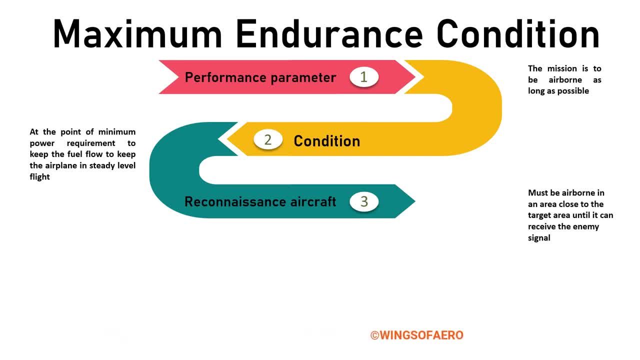 aircraft must wait, airborne in an area close to the target area, okay, until an unless it receives some signal, or in case of really aircraft, but also depending on the signal receiving from the commander, until and unless it don't relay or transmit the signal. similar case for the border. 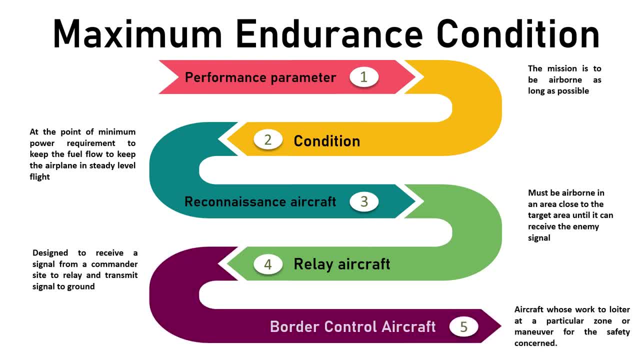 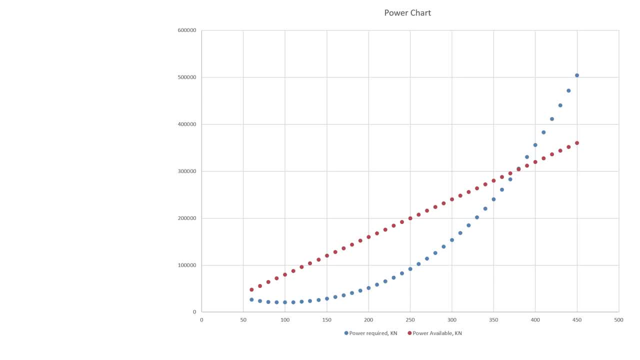 okay, or the most of the cases. the minimum power is also applicable, and then this conditions are obtained. also applied for an propeller driven aircraft. in this category, you need to plot a graph for an foreign power requirement and power available versus the velocity that will be observed. something like this, as I've 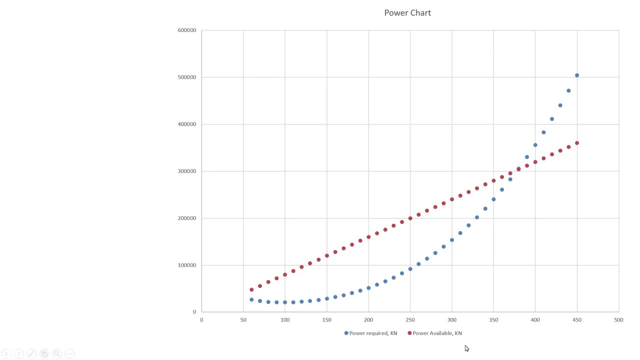 demonstrated, the aircraft should fly at an flight condition where the zero lift drag is one-third of the drag due to lift. so you have to apply this formula and then the velocity for an minimum power requirement can be find using this formula. you need to substitute here and L by D can be find again using this. 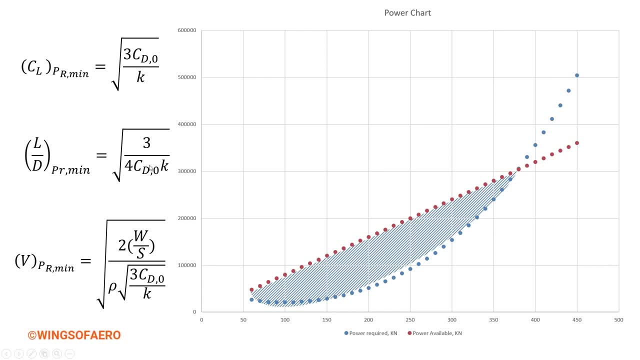 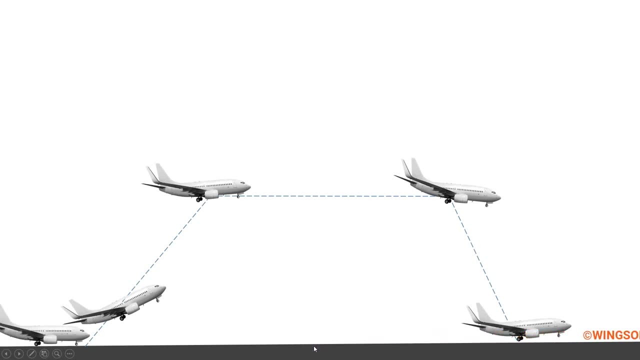 formula right now. finally, you need to formulate to estimate your range and endurance based on your mission profile, from the engine start to the shutdown. okay, now considering this speed, alt, your speed and theHHHH- ahhhhhhh, the altitude is constant during your cruise, so you need to use this formula for both range and 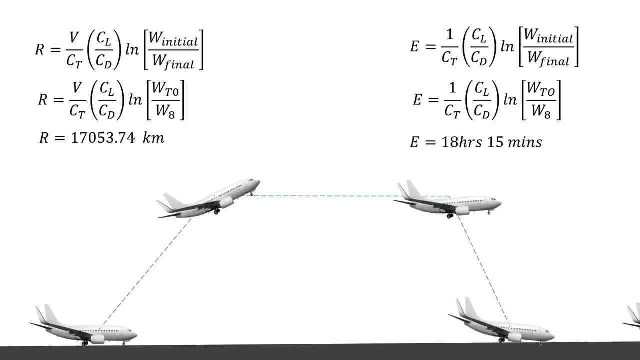 endurance. substitute into your following parameters and you get your range is about 17053.74 and endurance coming to be about hours and 15 minutes without refueling its fuel tank. so please make a note of one more thing here before designing. we have estimated that my design 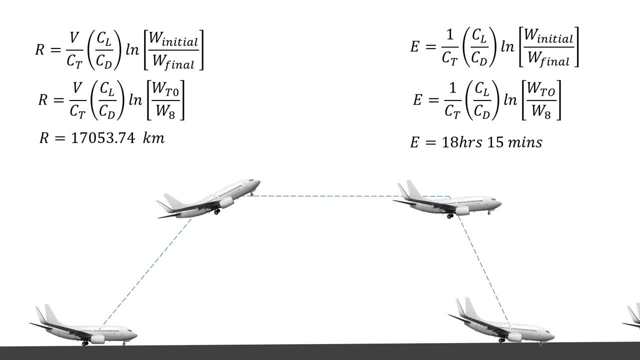 range. aircraft range should be around 15,000 kilometer and finally, when i'm finding out the performance, it shows that 17,053.74 kilometer. so it is exceeding the limit. you have to check that your range is exceeding or not. if it is exceeding, it's better, but in case if it is reducing from. 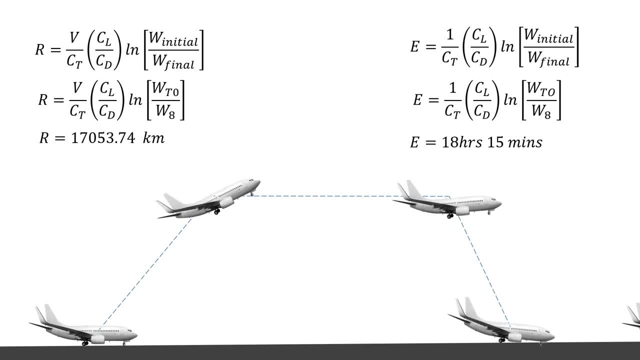 your design parameter. then again, you need to check where it has gone error. one more thing: make sure that your range is exceeding or not. if it is exceeding or not, then you need to check a note that, uh, this, this, this is a common standard formula and in case of minimum power requirement. 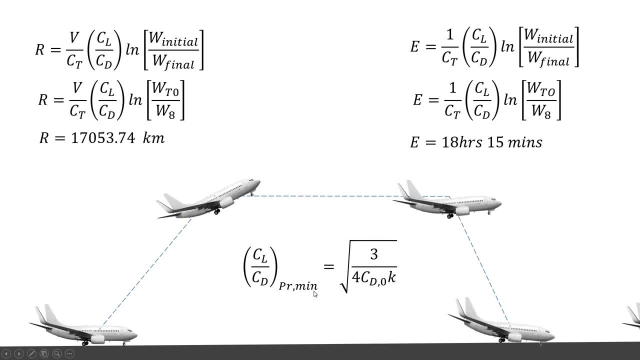 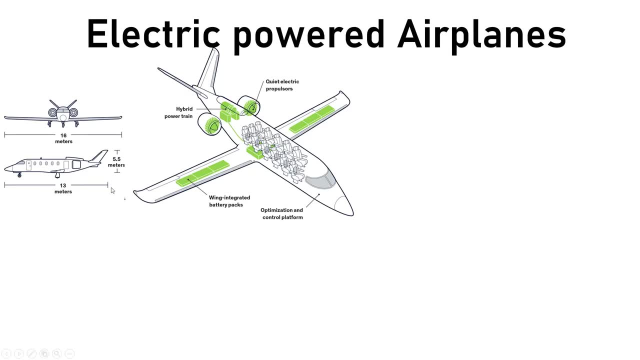 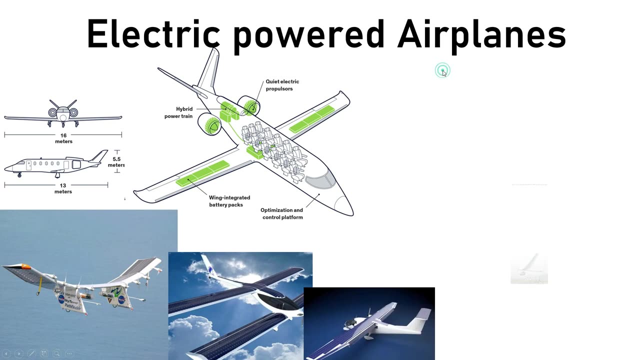 condition uh. to find out the clycd, you need to use this formula. this is for the minimum required condition. air airplane powered within solar energy are being developed frequently and a number of such airplanes are already flown, including a taxi with passenger. okay, now this electrical uh air. 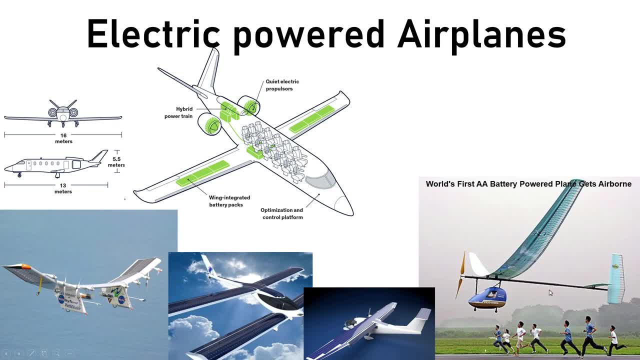 aircraft differ from this kind of fueled aircraft now is a different, is the weight does not change with range. so in such cases, uh, for such reasons, the brocade formula as for the range and the endurance, is not applicable. so rather, you will learn how to calculate the range of an airplane. 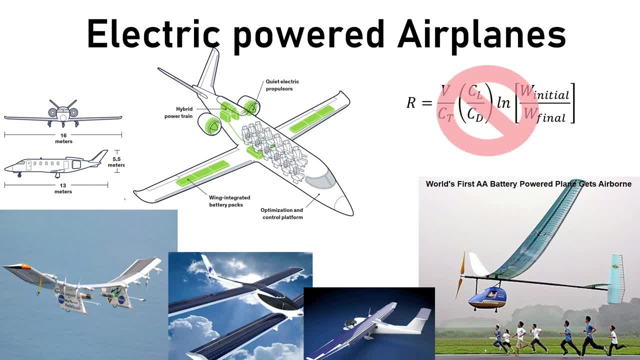 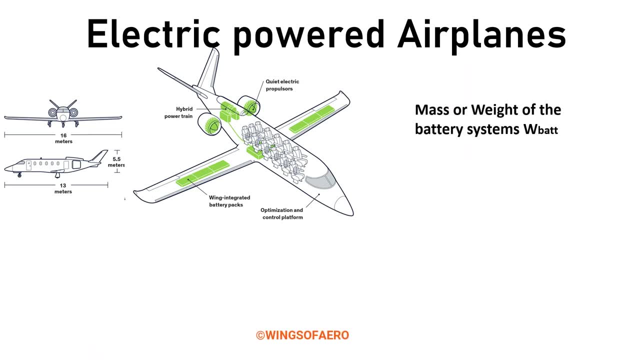 powered by electric motors driven by the batteries, assuming that the flight flies at an constant altitude. now let the mass or the weight of the air battery system be w b a t t. okay, and let that energy density of the battery is e bat, that is b a t t. now, then the total energy. 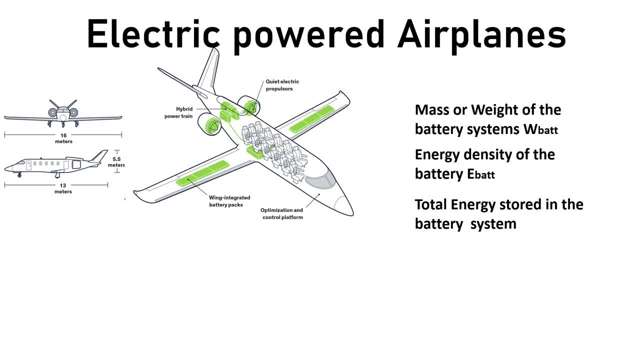 stored in the battery system will be capital e. so capital e equals to the mass into the energy density. right now, the power of the motor. suppose you have chosen some particular motor that is p electrical. then the time to run the motor, that is, to find out the. 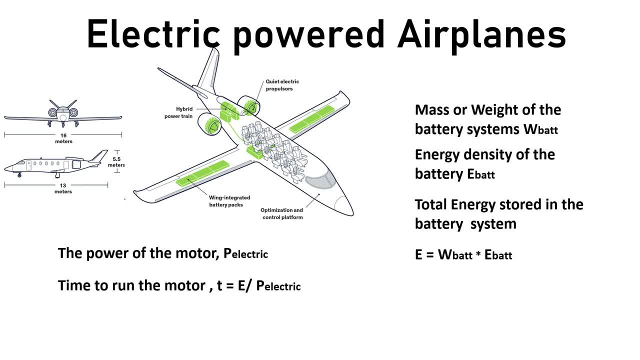 total time, or the endurance becomes the total energy by the power of the motor. so, like how, in case of electrical power, you can find out the how much time it will fly in the air based on the battery, based on the power of motor you're using now, after. 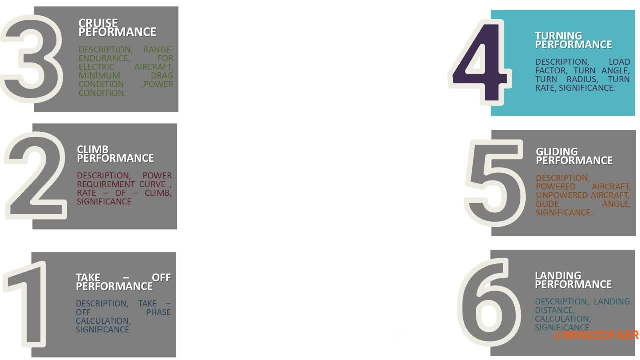 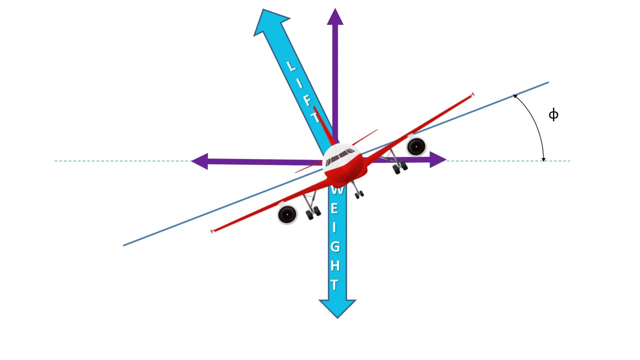 an endurance. one more interesting aspects of performance is a turning flight, whether will perform small turn radius or a small turning rate. so, recalling from a newton's third law of motion that any unbalanced force will accelerate a body in an direction of force, okay now the aerodynamic force that is tilted into a turn is a centipedal. 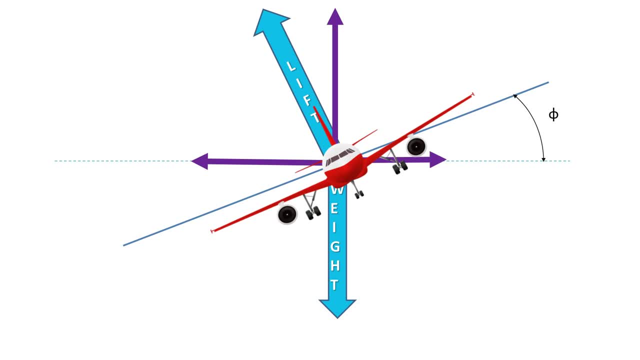 force. now it can be solved by the angle phi. a little trigonometry will be used in this figure right. so here the load factor equals to that, that is, l by w equals to the one by cos phi. phi is a banking angle, or by rearranging you can say that cos phi equals to one by n. 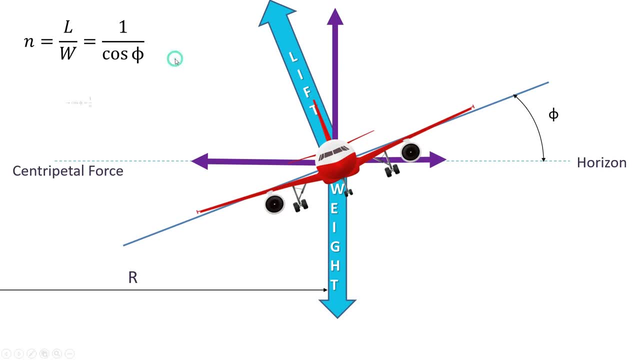 right now to find out the maximum load factor for your design can be applied. this formula, that is the tw by uh, t by w into l by d. applying that- and in case of my design it is coming to be about 4.8- is a maximum load factor. now for this particular load factor, what i will do is 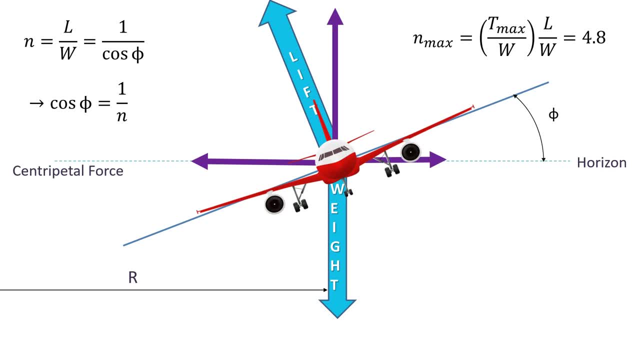 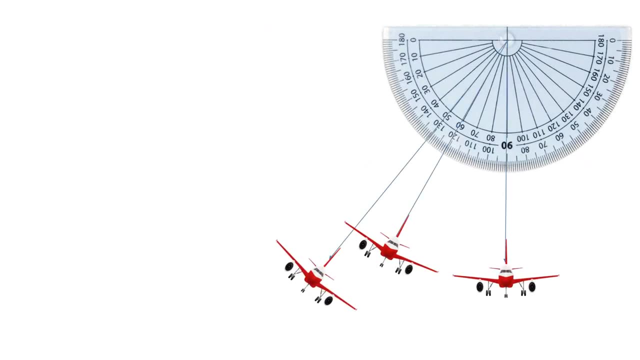 i will plot a way. uh, now, this is my maximum load factor, that is, the effective lift to the maximum weight right now. therefore, for in every degrees the banking angle based on the load factor will vary. for, suppose, 60 degree, the banking angle means a load factor will be of 2 or a 2g turn. 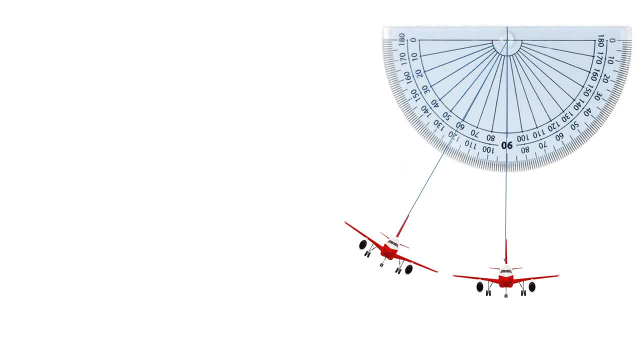 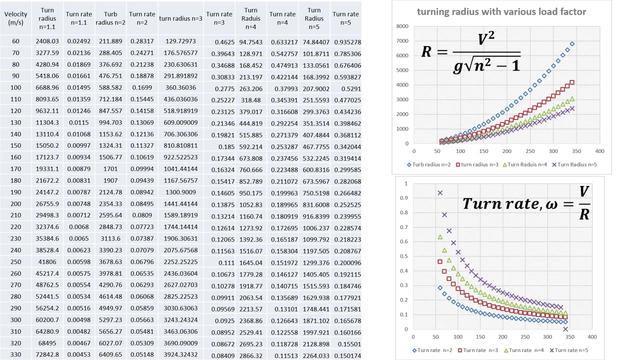 or, in case of level flight, is a 1g flight condition. now, based on this, two maneuvering indicators of performance characteristic of turning flight are turning radius r and the turning rate omega right. these two factors can be plotted against various velocities for your design. now, this is i have done for my design, and from there you can find out the maximum. 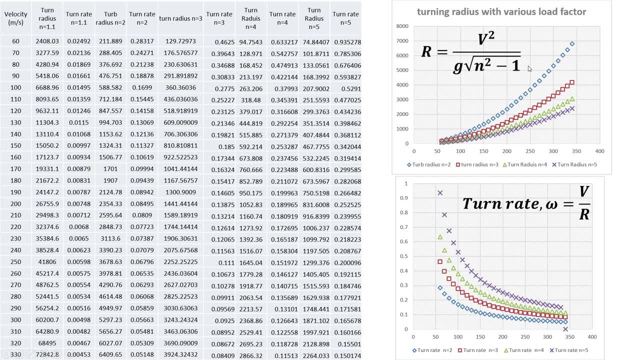 turn radius and turn rate for your formula, using uh for your design. based on this particular formula, turn radius in terms of meter and the turn rate in terms of radian. it signifies that turn radius is inversely proportional to the turn rate. okay, if the if during the turn radius higher will be the turn rate at a particular cl altitude load factor. 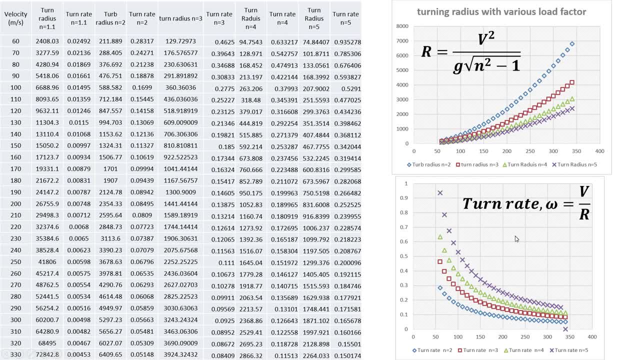 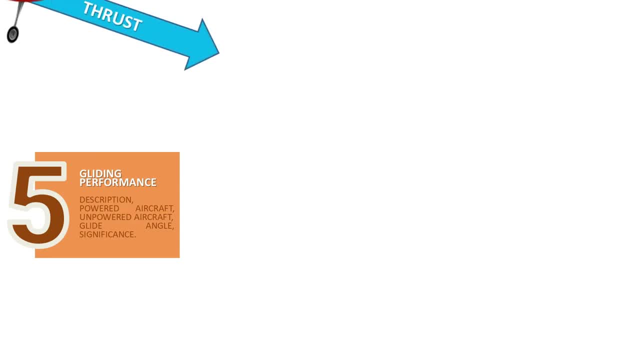 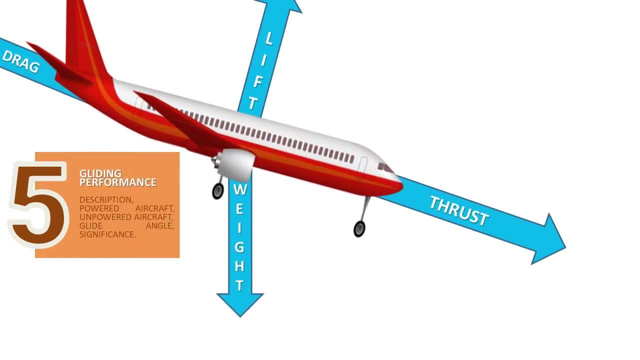 and the wing loading. so this is the significance of this turning performance: coming to the last phase is a descent and the landing so descent, and the initial approach phase of a flight starts at the end of the cruise phase and which the aircraft will start to approach for the landing for an 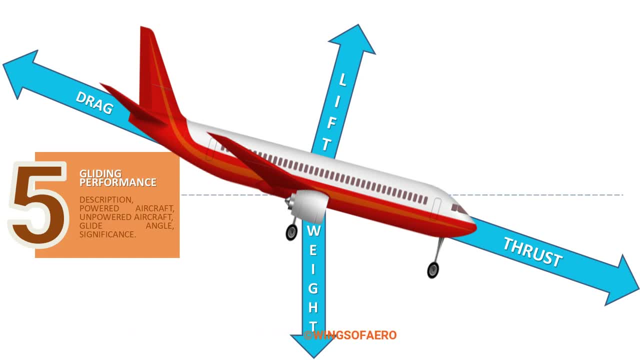 aerojet aircraft. so these are some major differences, as many of you guys must know, even if you are already working for a pilot or other business, or if you are already doing a powerful flight, or if you are working for a fully fueled robot now, during the departure and 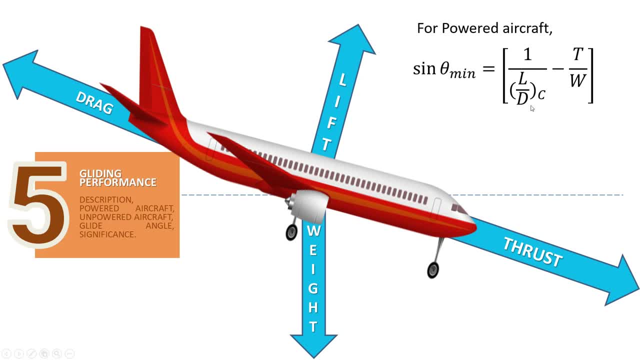 said powered aircraft. the analysis of gliding flight is essential for an standing point of safety. okay, so first we'll see that. power descent for power distant for in case of our design. so we have to use this formula, that is, sign in sine. theta equals to 1 by l by d, minus artists, t by w. now, uh, substituting the parameters, we get theta about minus 9.5. now, why minus? because it's different quadrant. when i will make set two hand aids, like a different squared approach and a soon getting made a FateWidel and all the points seinai, maybe get that angle throughout it, otherwise par. 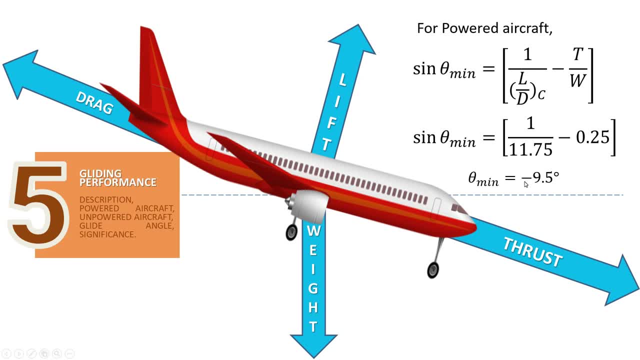 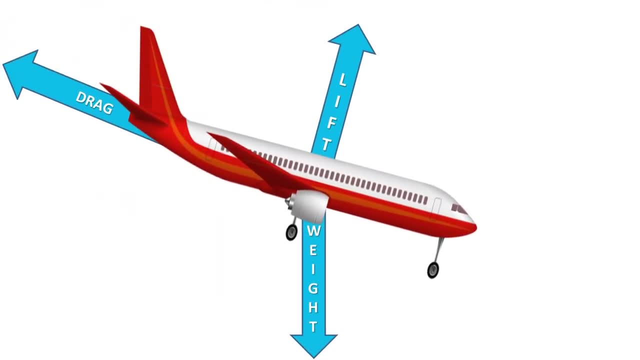 so that's why it is minus 9.5 degree. but in case of unpowered descent, like glider cell plane, you need to use this following formula: tan inverse equals to 1 by l by d maximum. so whatever your l by d, you just substitute and you will get the theta. okay. now, from here we can find out the best. 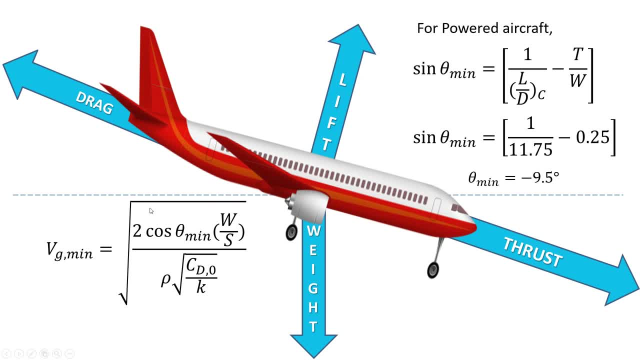 gliding speed at an equilibrium gliding angle can be calculated using this formula. now, based on this formula, you can find out your gliding speed, best gliding speed at what? during the phase of before the initial phase of landing. so you you have this formula and substitute values and, in case of mine, 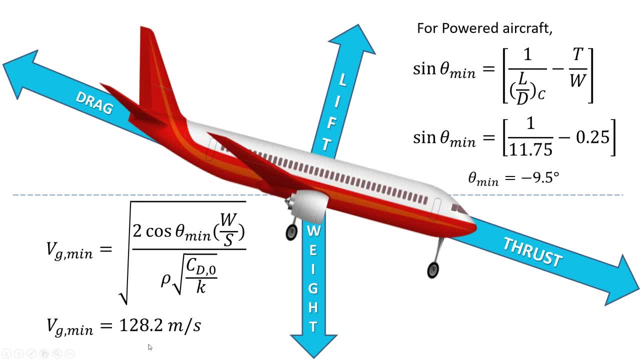 i got around um 128.2 meter per second. now, from here you can also proceed with your rate of sink if necessary. so, uh, mostly the rate of sink is very much necessary in case of gliding flight. so you can use this formula: that rate of sink equals to gliding speed into the sign of the. 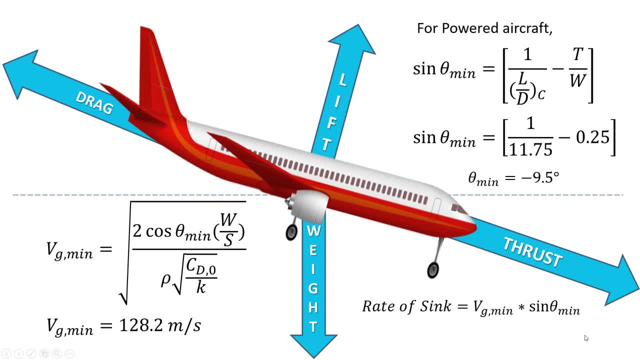 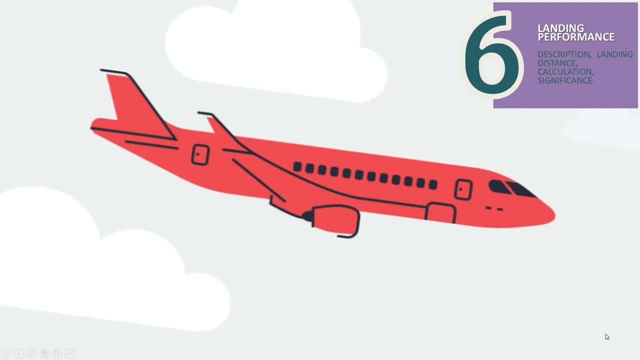 gliding angle. uh, so after substituting, you will get the respective value. now coming to us landing performance. landing performance starts with a descent and, depending on the engineering value of the glider, you can get the respective value of the glider. so you can use this formula. 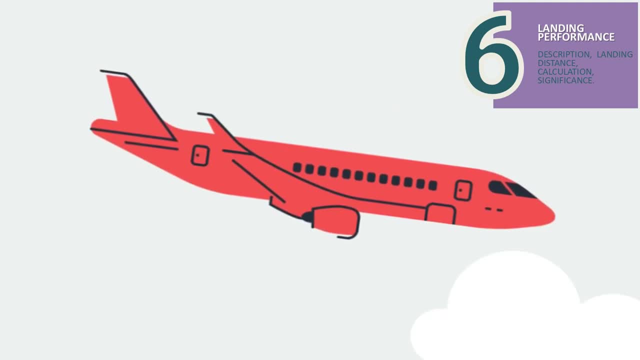 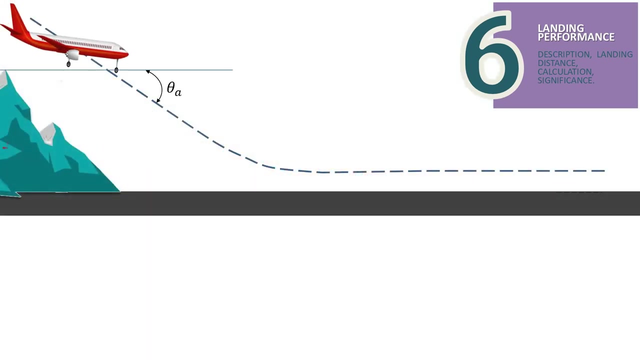 data and determine by the reference and the performance chart. now this minimum landing distance is obtained by the landing at some minimum or safe speed. it's a great challenge for the aircraft designer if approaches at higher speed. okay, so the landing distance is a distance from the point of approach until the engine shuts off, that is, velocity becomes zero. now the sum. 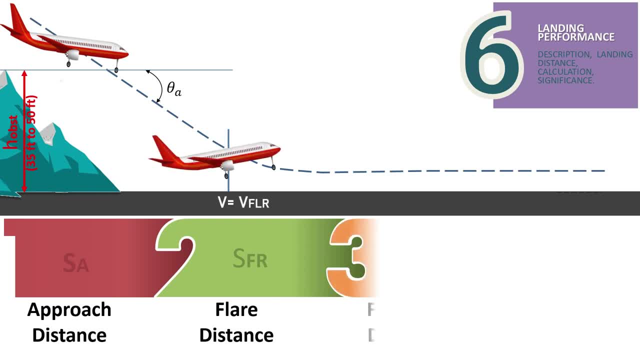 of approach distance, that is s? a, flare distance s? f, then the row free roll distance s? f? r and the braking distance s b? r. now the approach distance is s? a. that depends on the approach angle and the flare distance h? f now, according to all the engine take off and landing. it depends on the f? 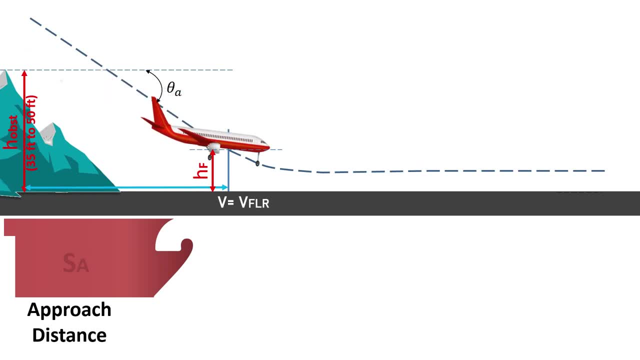 ar 23 and 25. the approach distance requires to clear 50 feet, that is 13 point, uh 15.3 to the 35 feet, that is around 10 meter distance. mathematically, this approach distance can be defined by 15.3 minus hf by 10 theta a. hf is the flare height and 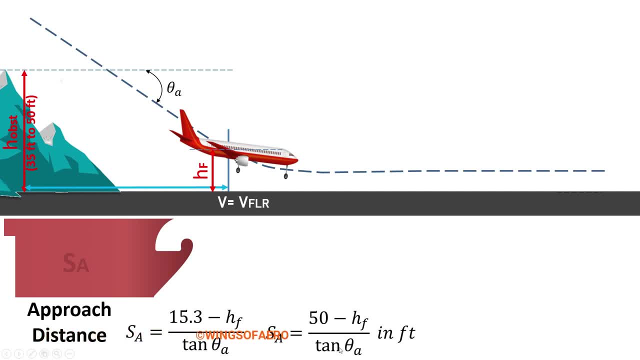 theta a is the approach angle in terms of meter and if, in case of fit, you have to get 15 point3 f and this approach distance can be found by 15 point3 minus hf by tan theta a, hf is the flare height and theta a is the approach angle in terms of meter and if, in case of fit, you 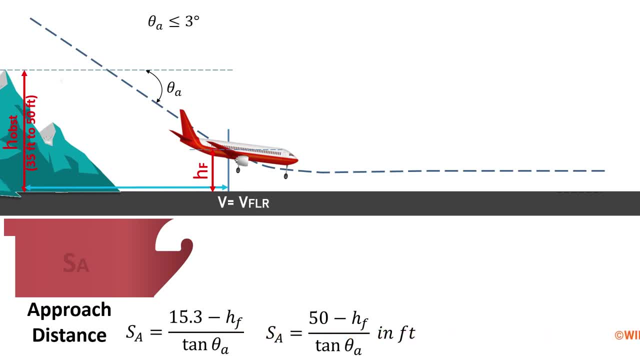 you have to use this formula now, based on the equilibrium flight condition approach, angle is should be small, equivalent to 3 degree. let's consider 3 degree now. the flare height can be find using this formula, and r is the rate of turn radius during landing. now turn. 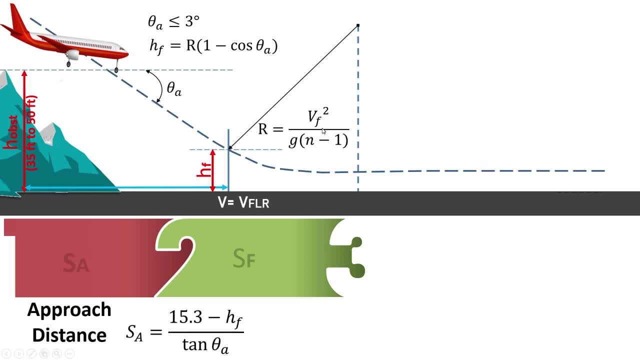 radius during landing can be find using this formula again: vf square by g n minus 1, vf is the flare distance, flare velocity. now the path, the path radius during flare are vary from aircraft to aircraft. now it has to be considered again based on faa regulation. now 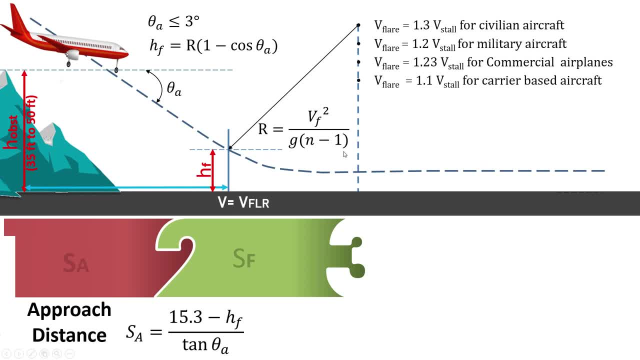 the flare distance. it varies as you can see. in case of my design, flare velocity equals to 1.2. 3 of stall velocity. now applying the value, we get around 74.32 meter per second. now, same the load factor as of take off, that is 1.296. now substituting back in this respective formula: 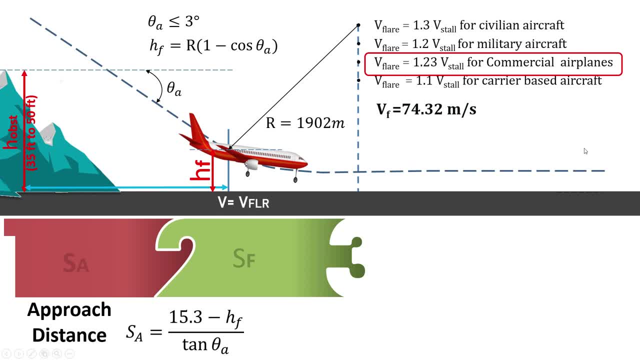 we get that ah turn radius about 1902 meter. therefore hf becomes, after substituting the values, that is 2.62 meter. now, substituting all the values in sz- that is the approach distance- we get 15.3. minus 2.62. by tan 3 degree we get 2.. 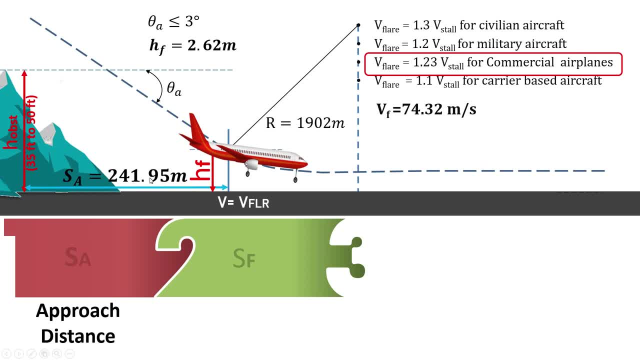 241.95 meter now. flare distance sf can be calculated using this formula: where ah flare, ah angle and a approach angle consider to be same. now again, substituting the values in this respective formula, we get the flare distance about ninety nine point five, four meter. right then, in particular. we are going to calculate a flared par happened as a Dodge Mane, инструмент f. f can be calculated usingương orbyste. h goes the approximately approach formats that are considered to be same, and it is meant for both the curves of aIPR, aPANK. 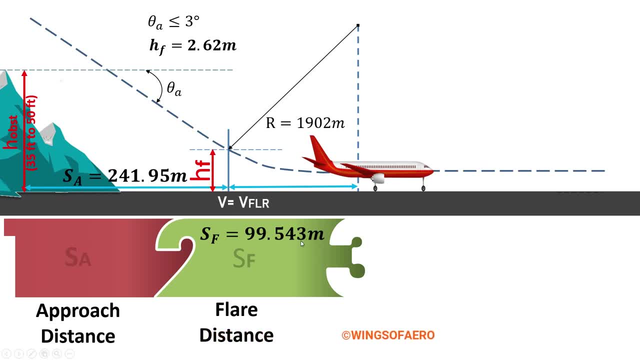 buraya instruments with which we can find out that the particular foods that are needed D in the smoketiris that are present in the fragoraor that are used are personnel speed and 아이renreacts. now the free roll distance is determined in a similar way as a takeoff, like for in case of small 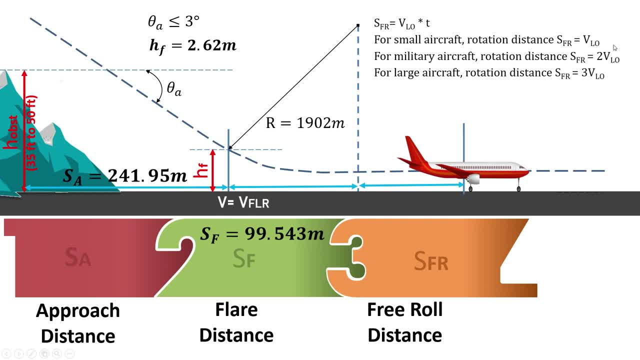 if sfr equals to 1, 1 into v landing velocity and in case of for a large aircraft, sfr equals to 3 into v of landing velocity. now, whereas landing velocity is 73.23 meter per second, and substituting for, in case of my design, that is large aircraft, that is 3 into 73.23, coming to be about to 19.69. 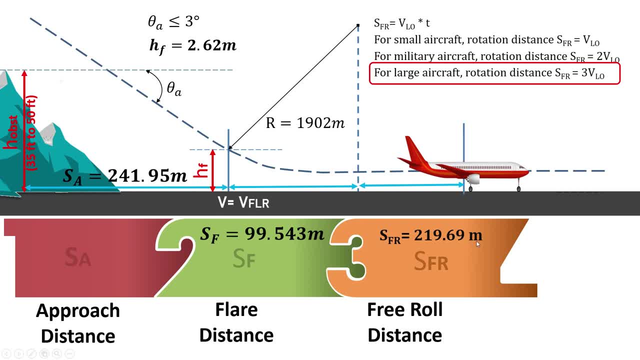 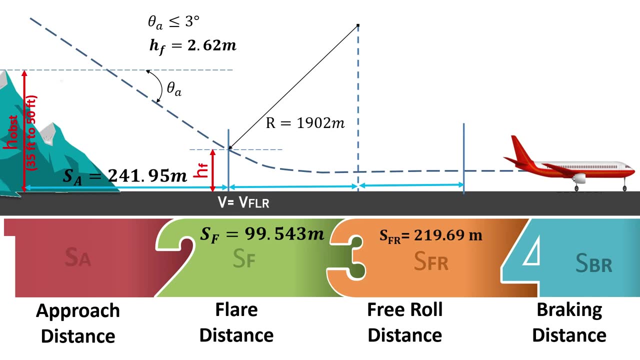 meter. now, finally, determining the uh, determining the breaking distance, that is a sbr. the last phase of our design can be estimated using this formula. now here, what happens when we are applying the break? it is no more accelerating, but it is a returning. so that's why the 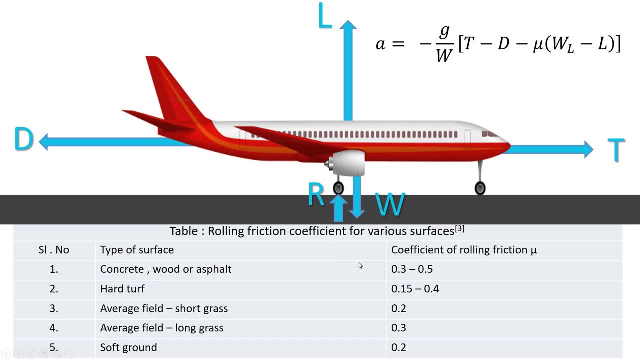 a is considered to be as negative. so again, substituting on this particular formula. now here, another factor will play a key role. that is a new, now mute. when you're applying a break on this particular surface, that is uh, what kind of coefficient of friction will occur that has? 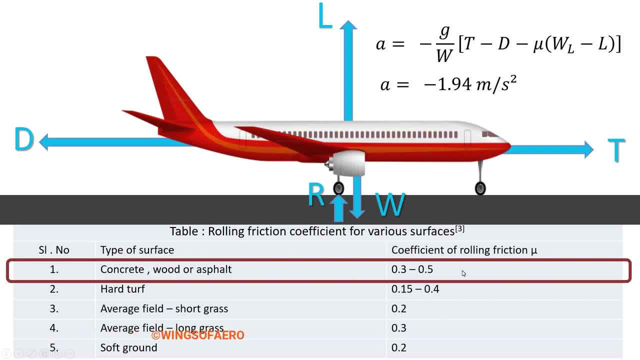 again has to select from this table. now, in case of my design, i'm going to choose. i have chosen. it is a concrete, that is, mu becomes 0.4 while landing. so, uh, one more thing: keep in mind that when you're substituting this particular formula, you have to consider the take of weight of the aircraft during landing. 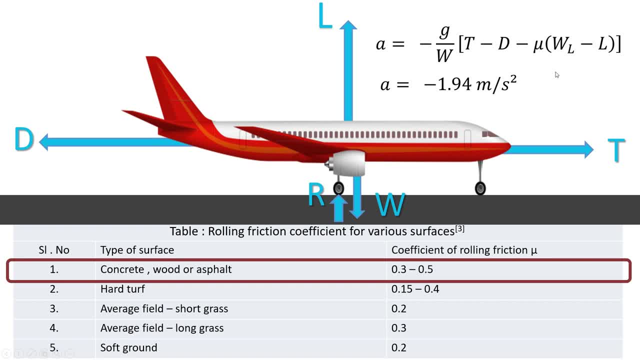 so during landing, the weight of the aircraft was 276610.983 newton. so these are the values during the particular phase of lift, during landing and drag, during landing. these values need to substitute- and we can find this, uh- recurrent values and again substitute back to this particular. 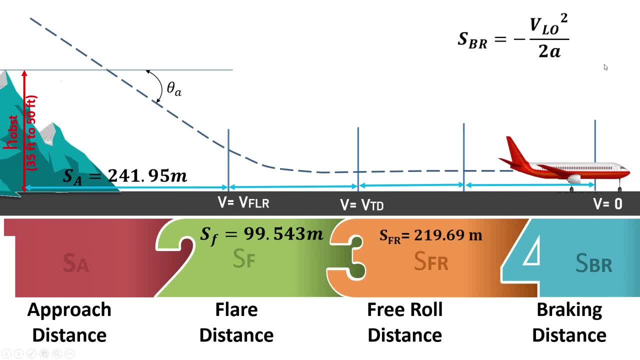 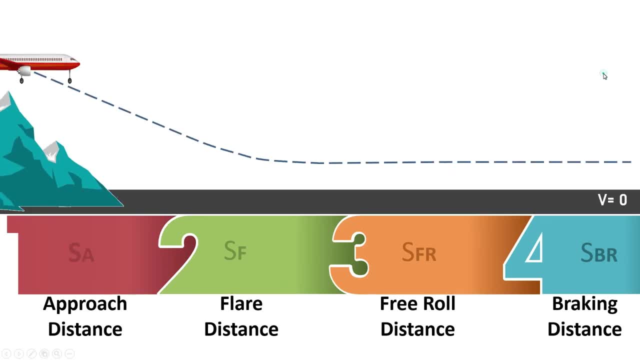 formula of sbr. that is a breaking distance and we get around 1382.25 meter. so from here we can sum up all the three or four parameters to find out the total landing distance, that is sl. so sl equals to sa plus sf, plus sfr plus sbr. now, when you are, 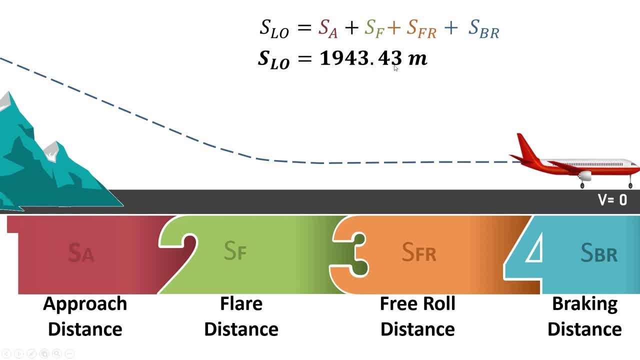 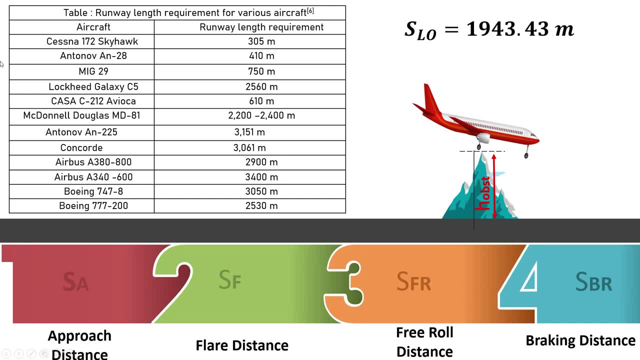 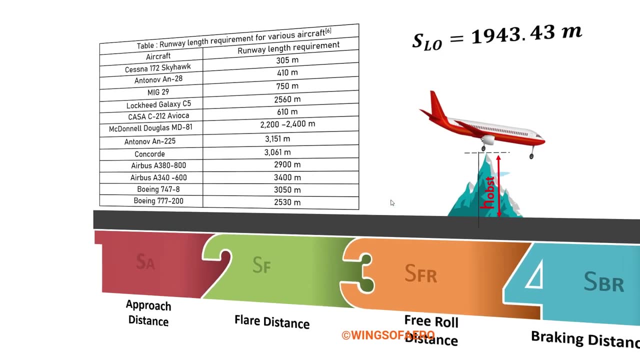 applying all those values again, you can get around one, nine, four, three point, four, three, three meter. now, referring again, referring back to this uh takeoff and landing distance for boeing and airbus. again it seems to be really less value and from here we can bring to a conclusion that